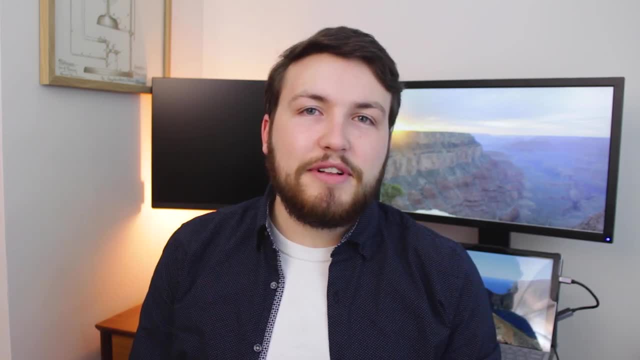 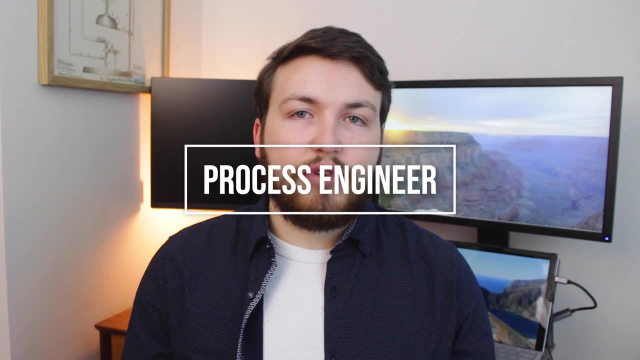 Hello world Eggs. here. Today I'm going to talk about my favorite chemical engineering roles and how to get into each of them. First and foremost, I think the most common role for chemical engineers to take on is the process engineer. Process engineers I've talked about in the past and it's usually what I talk about when I talk about chemical engineering. 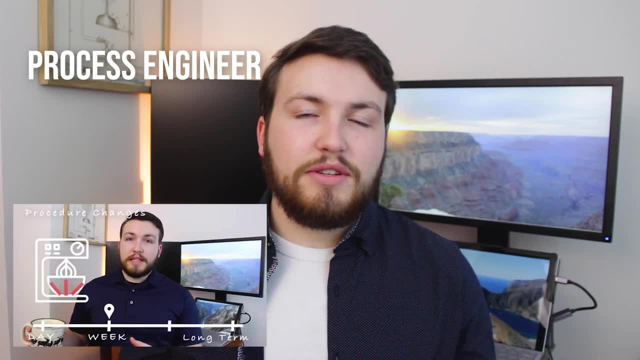 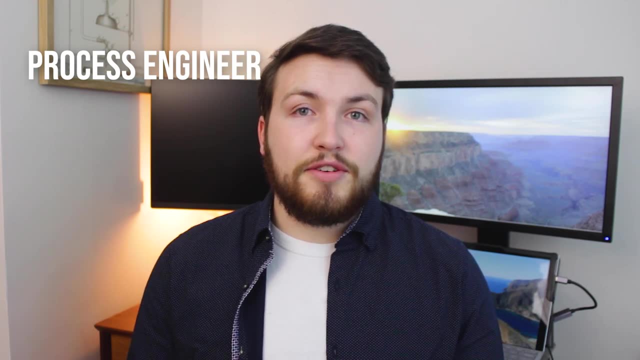 I even made a whole video about it in my Day in the Life video, and I go into a lot of detail there. so check that one out if you have the chance. Process engineers could be at either the beginning of their career or at the end of their career. 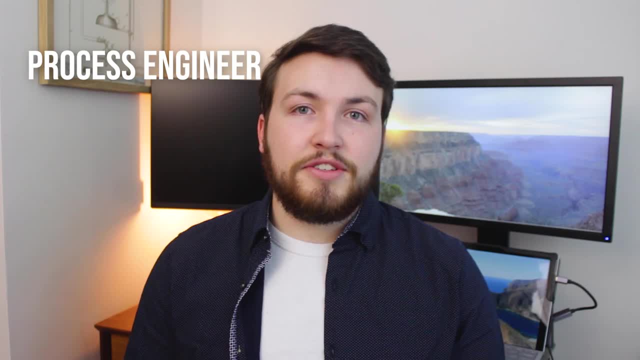 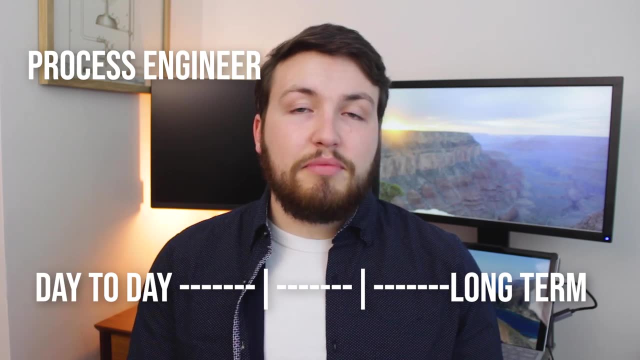 You can have really, really new engineers or really seasoned senior engineers working this job too. Process engineers can either focus on day-to-day real-time troubleshooting or long-term improvement projects and implementation of new technology, Or any combination of those two things. 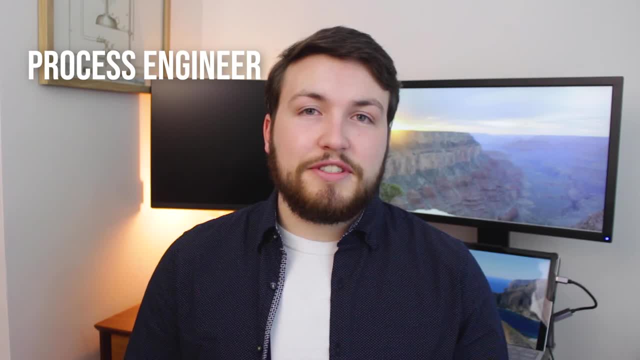 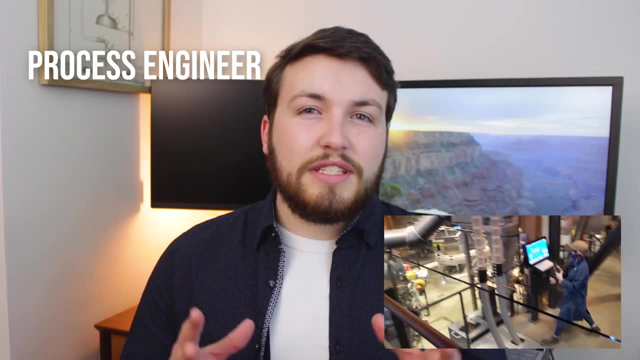 I think that process engineering is the best manifestation of the chemical engineering skill set. You really get to focus on the big picture process at any given chemical facility and you get to really focus on the in versus the out, the different chemical changes and thermodynamics. 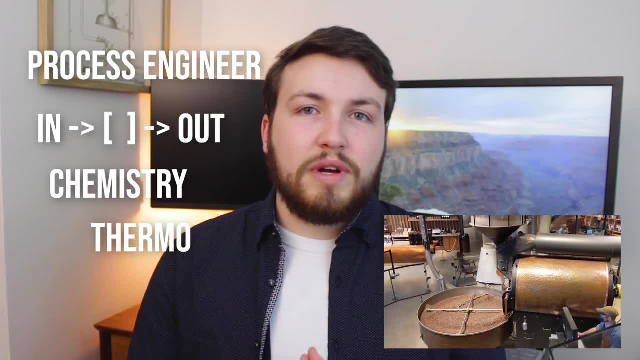 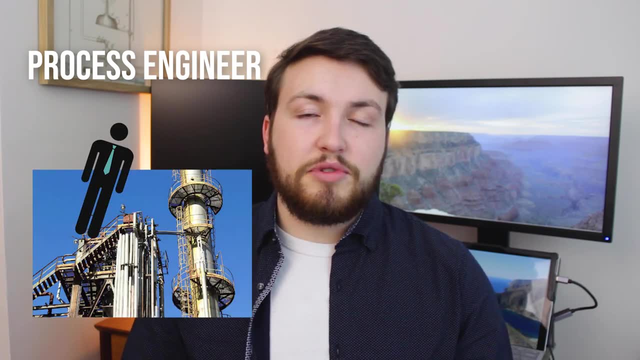 the specific interactions that might be happening in that process. You're really focusing on what chemical engineers are trained to do As a job process. engineers are really just supposed to be a technical expert on a very particular part of a chemical process. As a technical expert, they can understand how exactly to manipulate the process. 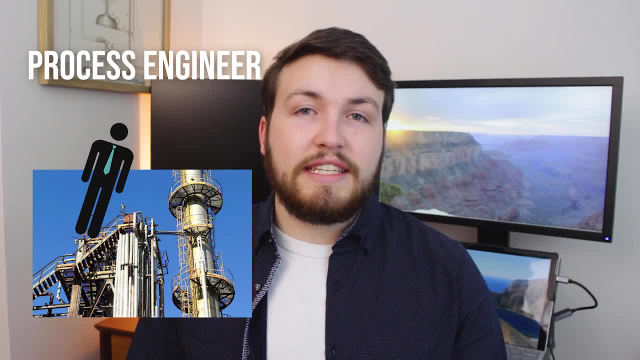 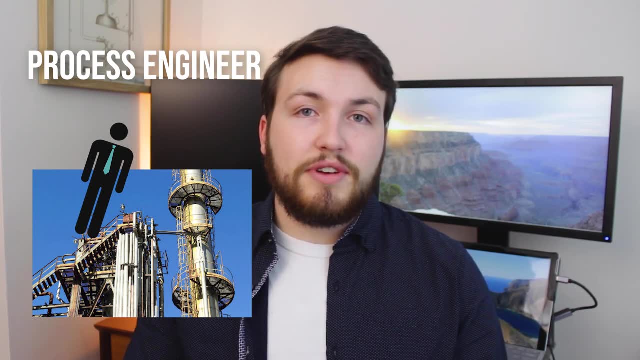 and make it change and be more productive, more safe, more effective, Or they can better investigate issues that are occurring and try to find ways to solve them. At the end of the day, anyone can run a chemical process if properly trained, But not anyone can change a chemical process or start up a chemical process. 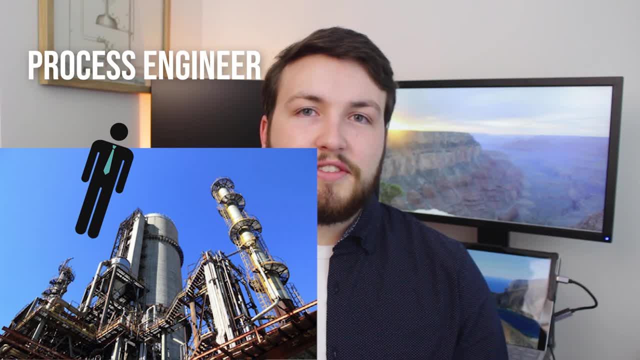 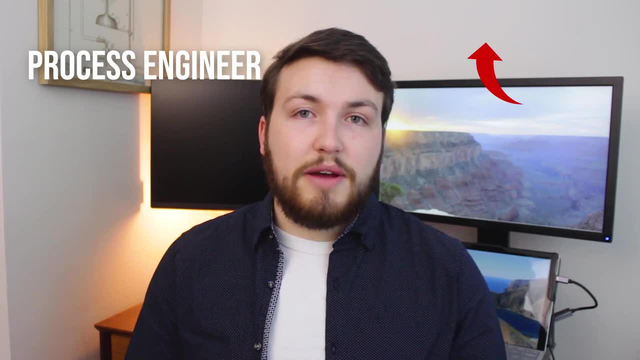 in a way that's most beneficial to a company, And that's where process engineers come in. If you want to get into process engineering, the best way to do it is to just follow this video I made here talking about how to get a chemical engineering job after graduation. Most companies will try to start off their chemical engineers in this role, And I think that process engineering is a great place for any new chemical engineer to start at, because it kind of exposes you to all of the different roles that are involved in a chemical facility. 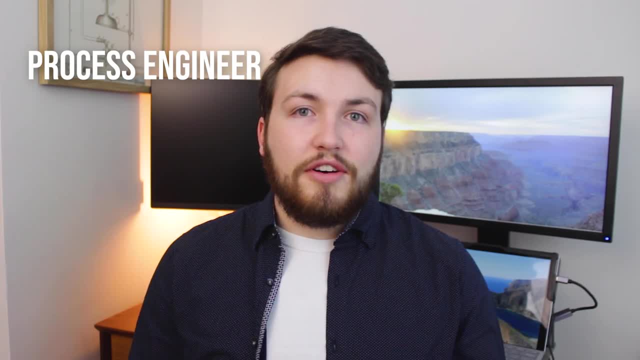 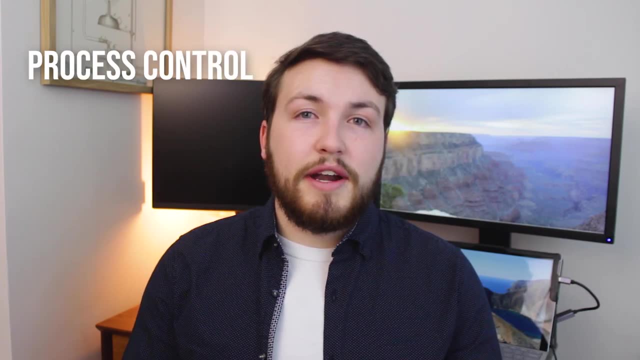 and it gets you kind of into, or at least involved with, all these different areas that I'm going to get into next. So let's get into some of those other roles. One of my favorite is process control and automation engineering. This is probably one of the fastest growing, most interesting chemical engineering roles right now. 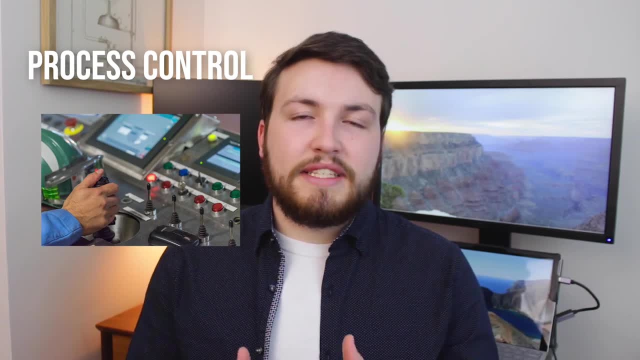 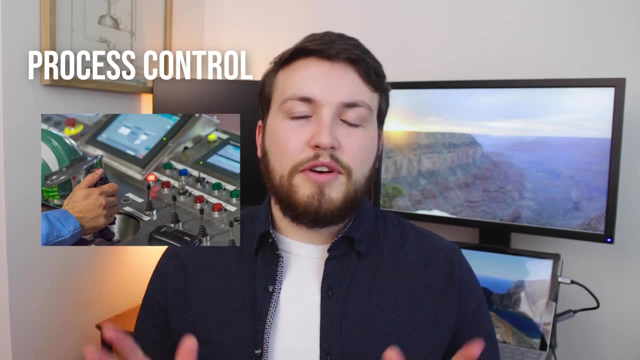 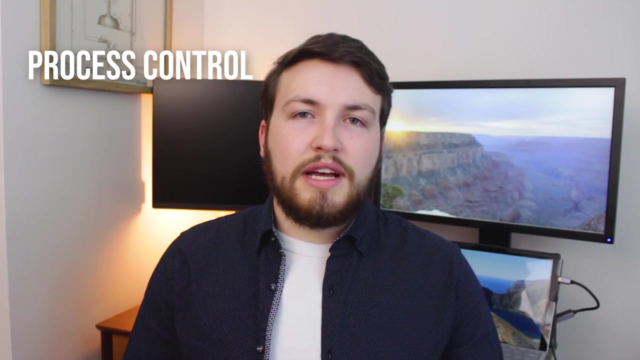 And it's basically following this giant boom of the tech industry. I've talked about it a lot in my coding video, among other things, and I've always said, oh, process control, process control. you know, look over there. But in general, the process control engineer is focused on the automation of a chemical process. 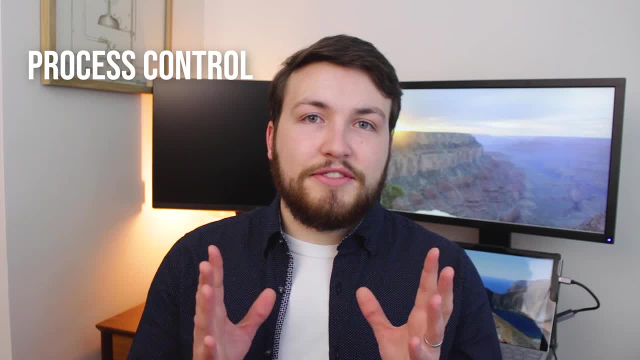 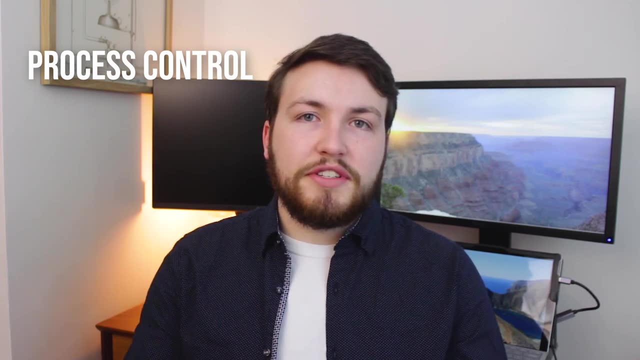 through computers and IT. There's no such thing as a chemical plant that is fully manual. It's all automated. Majority of chemical plants are extremely automated through different computers and different controllers that allow you to make a consistent product in the end of the day. 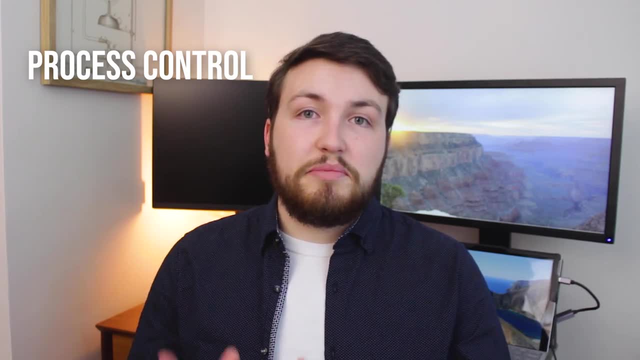 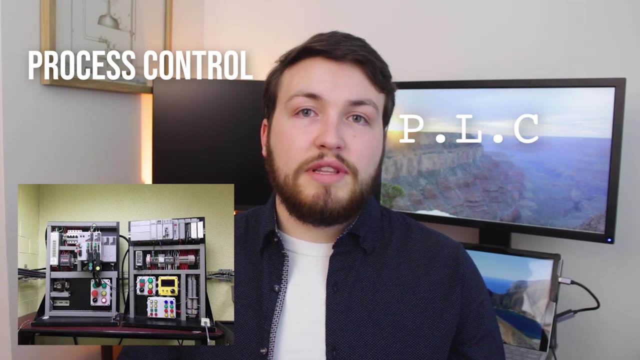 Usually automation and process control engineers will either focus on PLCs- programmable logic controllers- or the DCS, the distributed control system. The PLC is more for low-level process changes, sort of like turn this pump on, turn this pump off. 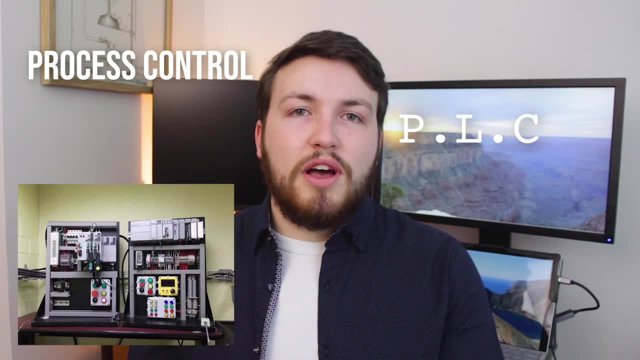 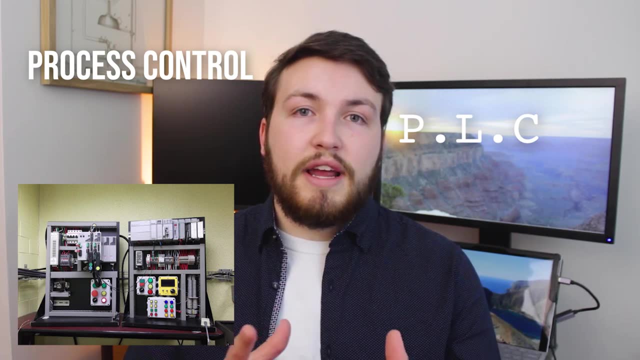 The controllers are usually slightly closer to the process and maybe a little bit slower, maybe a little bit less logic involved. This is a role that's often taken up by electrical engineers as well, because there's a lot of computer and electrical components that you have to mess with. 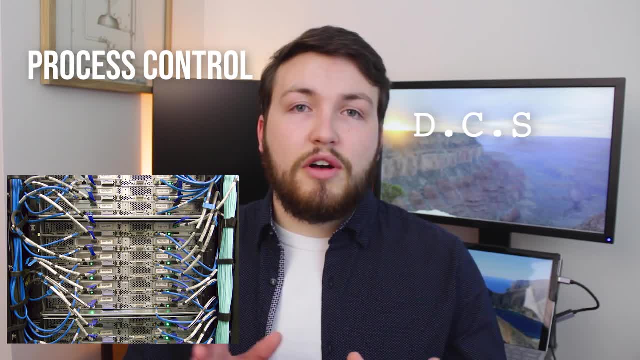 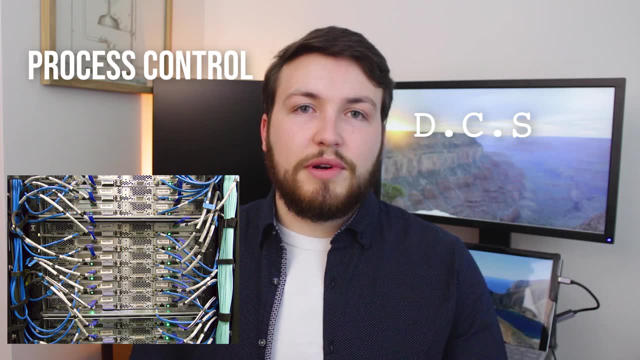 The distributed control system is sort of like the brain or the ultimate computer behind a chemical process. that's more complicated. Sort of a step back from all your different controllers and instrumentation components When you see a control room with a bunch of operators working on all these different screens. 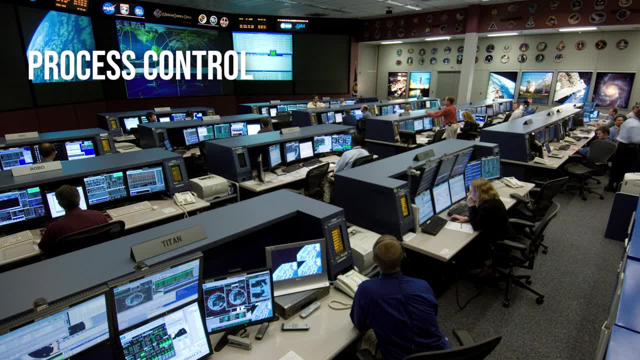 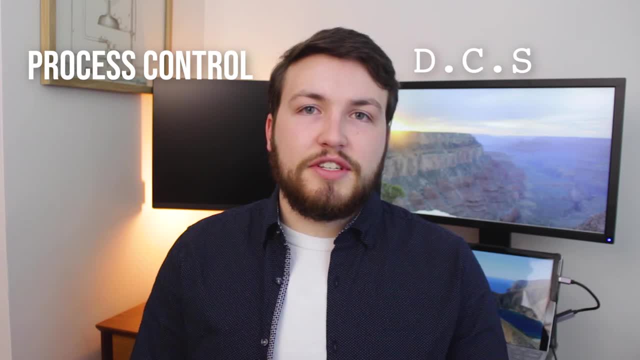 they cover a whole room. There's like a circle Or like a NASA launch team staring at computers in a giant room. That's sort of a visual of the DCS system that process control engineers might modify. The DCS system does a lot, but it mostly just allows operators to interface with the process. 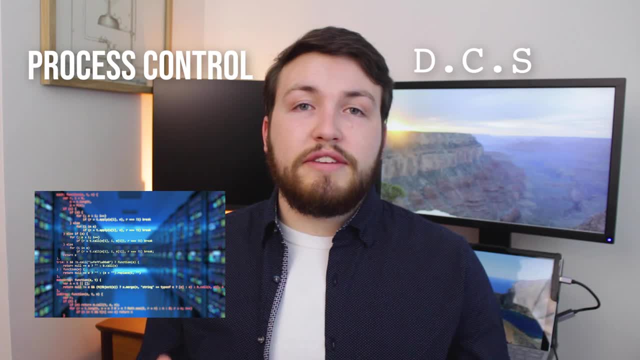 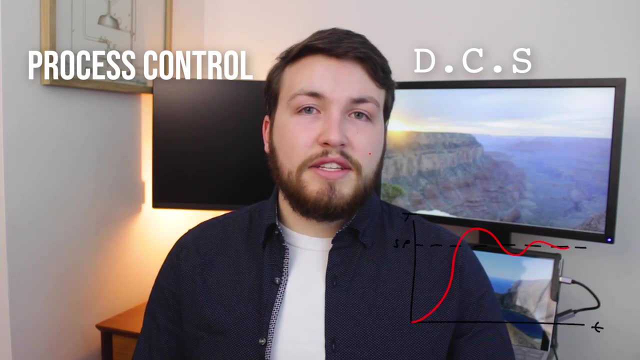 and control it from a computer. It also controls for all the different process steps that can't be done manually. One example is increasing the temperature in a tank with steam. It sounds like a simple task, but if you want to get to an exact temperature by adding steam, 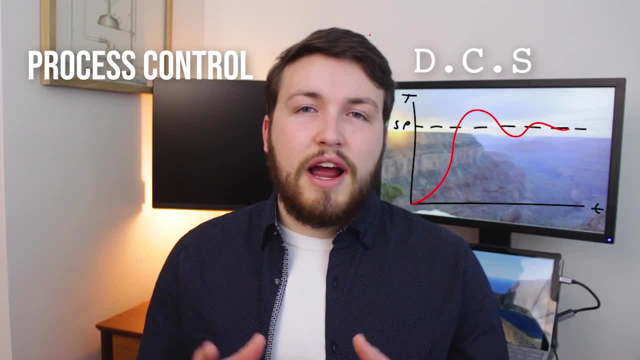 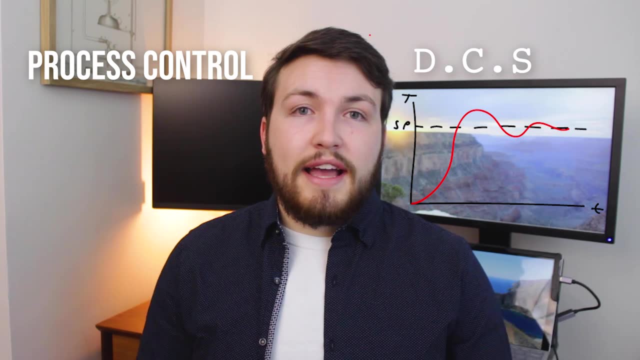 it can get pretty complicated pretty quickly. Your DCS system needs to account for how much steam should be added, how quickly, and not have too much overshoot or fluctuation. Now, if you can imagine controlling for a chemical reaction such as polymerization, 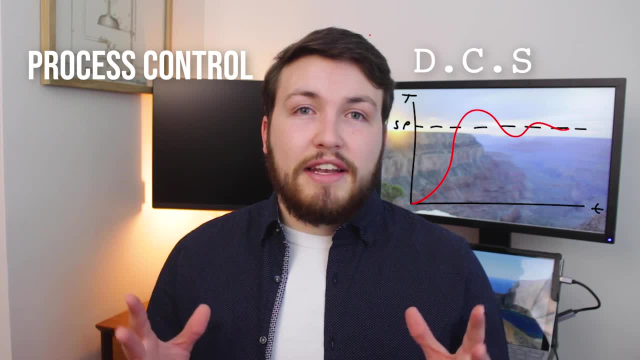 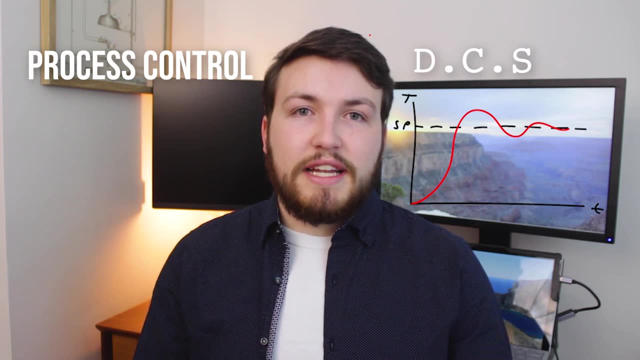 it can get a lot more complicated, because now you have not only this heat that you're adding, but you have a certain flow going into the process and all these different monitors that are telling you temperature and pressure changes that have to be controlled throughout as well. 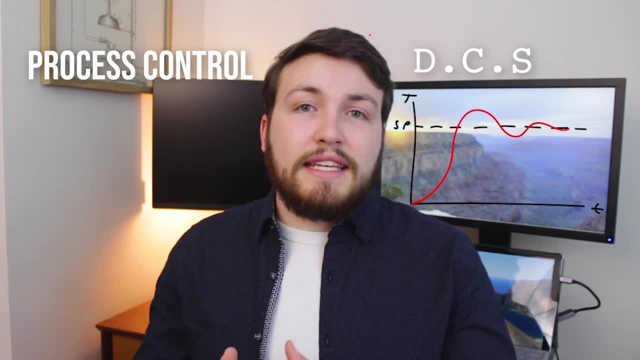 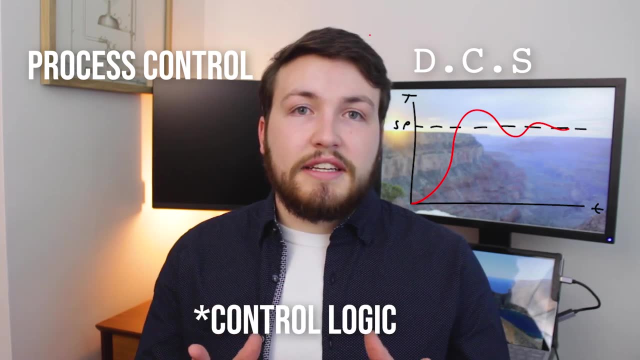 These control systems require a lot of different functional skills like IT and programming, but at the end of the day, the reason chemical engineers are so desired for this role is because they require logic, the chemical engineering logic, to allow you to understand exactly what happens. 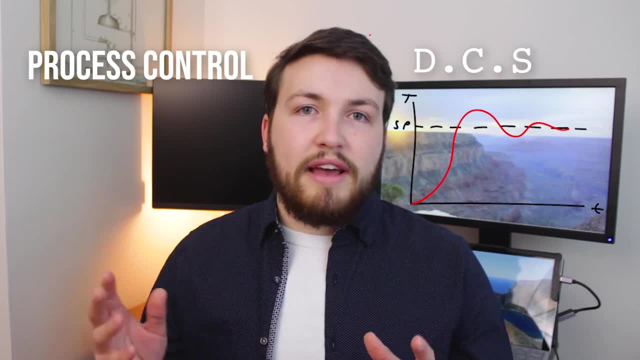 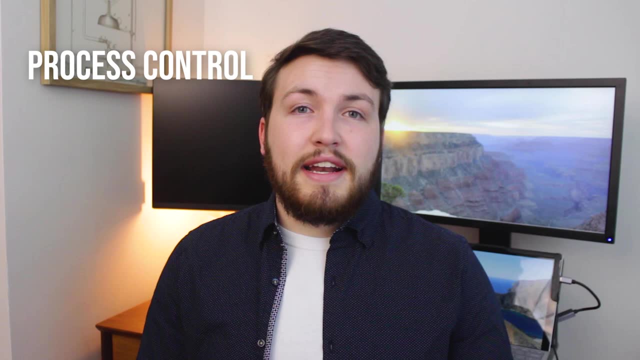 when I add this temperature to this reaction and what happens when I have this type of flow going to that reaction. All these different things are chemical engineering problems. It takes a really skilled chemical engineer to find out how to design a control scheme and program it in such a way that it saves the company the most money. 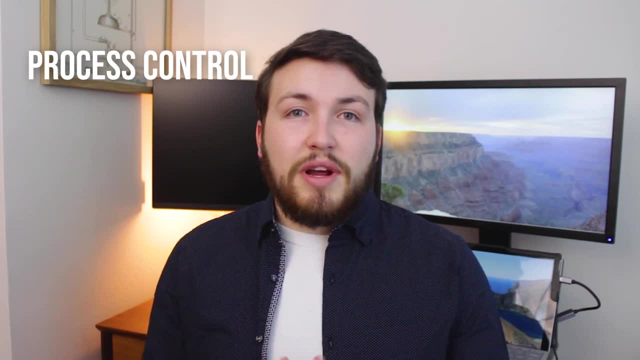 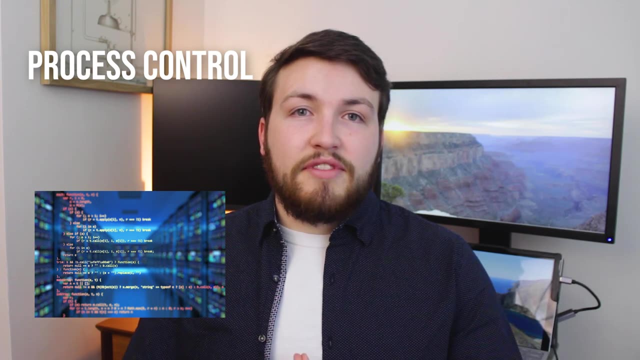 and causes the least amount of safety issues, etc. etc. Process engineers also deal with a lot of data. They do a lot of data management and data organization, which is why they benefit a lot from this whole big tech, big data boom that we're talking about. 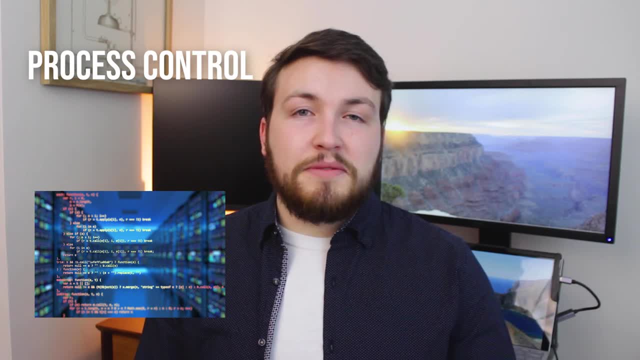 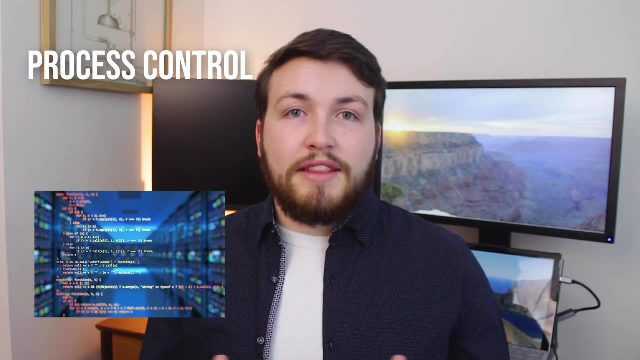 Computer technology, like hardware and software systems, as well as AI and ML, are growing really, really fast right now And there's a lot of opportunity for process control engineers to take those technologies and implement them into a chemical process to save the company tons of money and really really improve the chemical process. 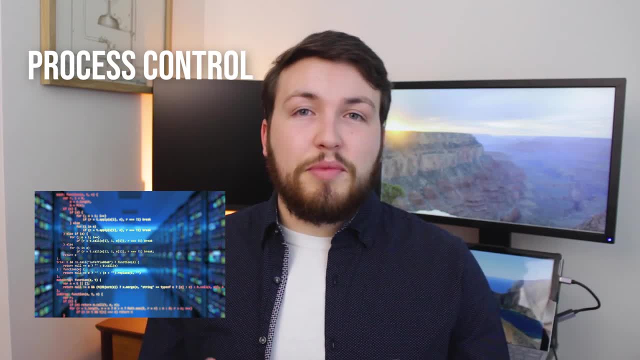 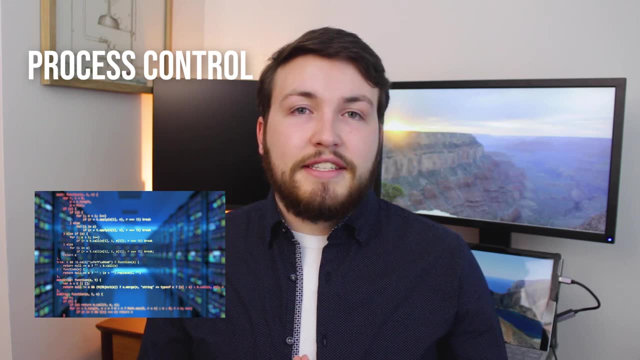 Because of all that opportunity. there's a lot of companies that are hiring more and more automation and process control engineers to take advantage of it. If you want to get into process control and automation engineering, the best way to do it is to start off as an intern in one of those roles. 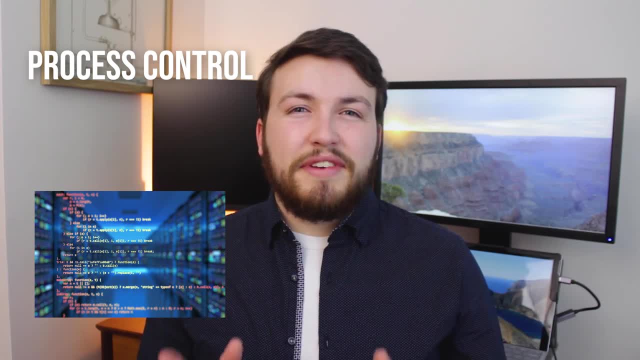 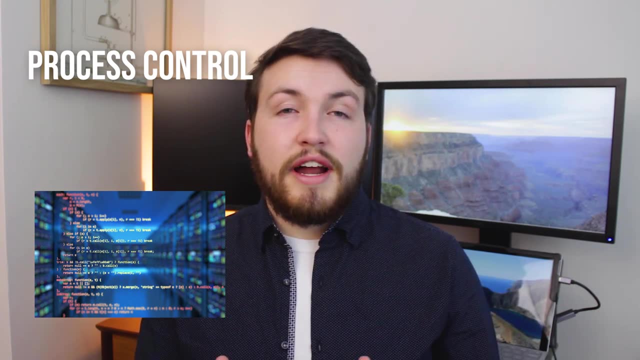 at a company that focuses on that sort of work. There's a lot of different certifications you can earn, depending on the industry and the type of work you're getting into, but you're mostly going to want to focus your experiences on process control, automation, IT programming and controllers. 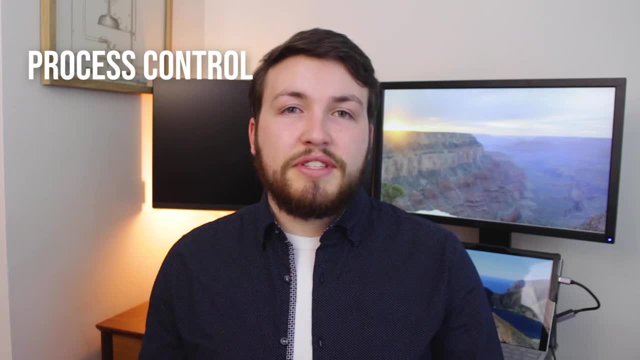 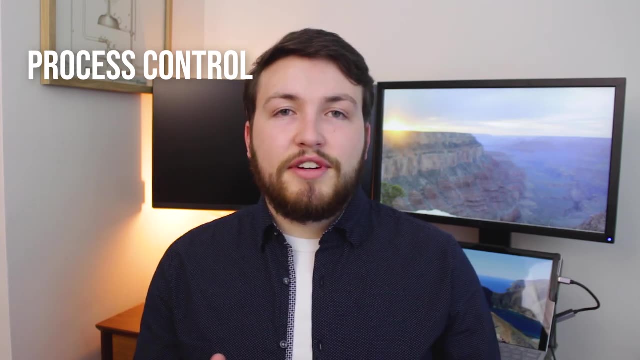 With enough background on either the software or the hardware side of things, you shouldn't have too much trouble working your way into a process control job as a chemical engineer. Depending on your setup, it could either be your first job or something you do after a few years of process engineering. 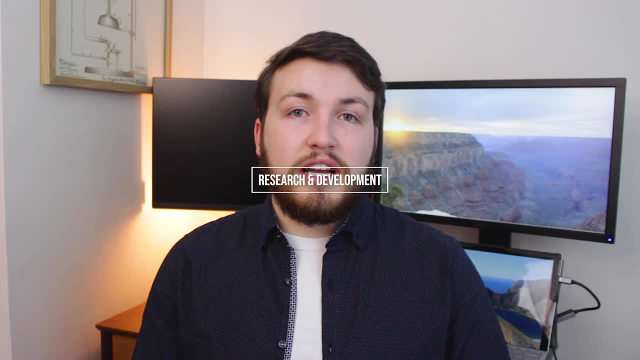 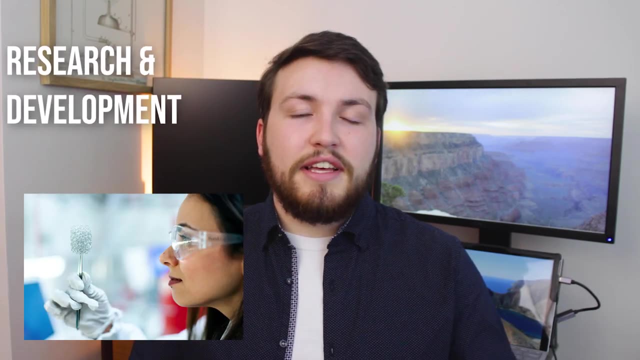 It's really exciting and it's a lot of fun to be on the cutting edge. so let's talk about R&D and product development engineering. Product development engineering is really fun because you get to work on new products and you feel like you have an impact around the world. 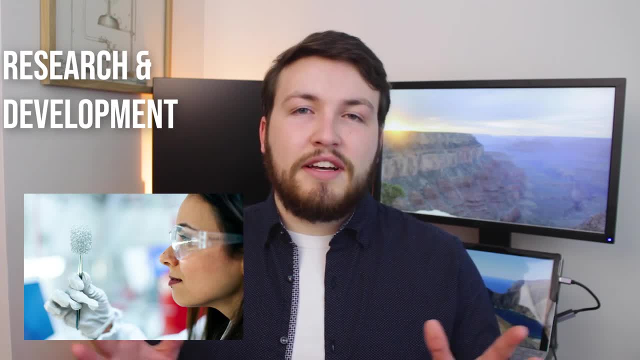 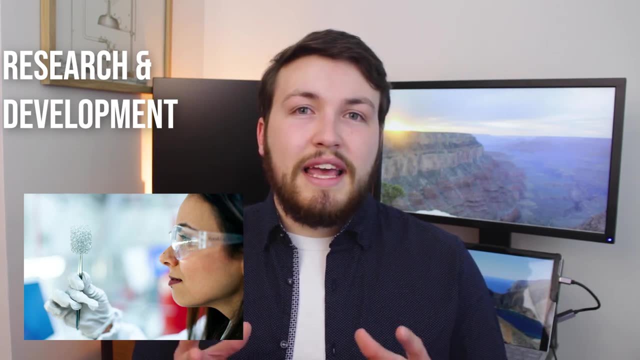 and it feels like you put a piece of yourself into this new technology. If you're working as a process engineer, improving a process, you're having an impact, You're making it more efficient, safer, more environmentally friendly, but you're not really changing the process. 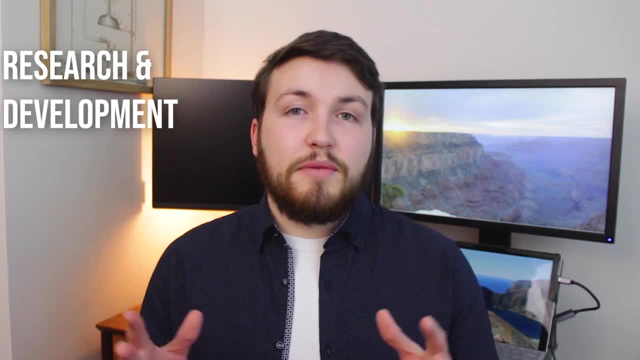 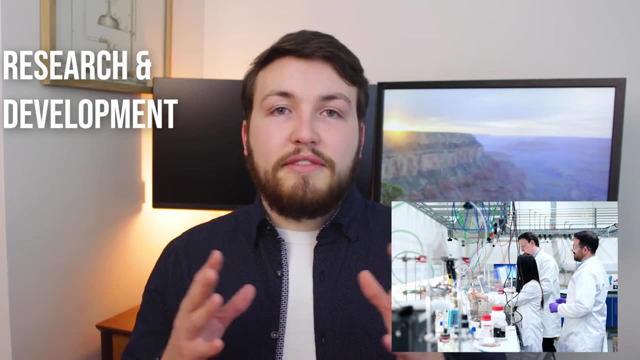 Product engineering and R&D are a lot different from your manufacturing jobs, because you're working on projects that are developing new products, You're doing a lot of testing, you're doing a lot of market research and you're trying to fit some new market need. 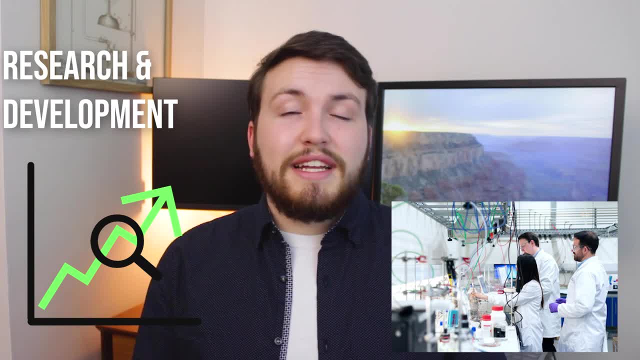 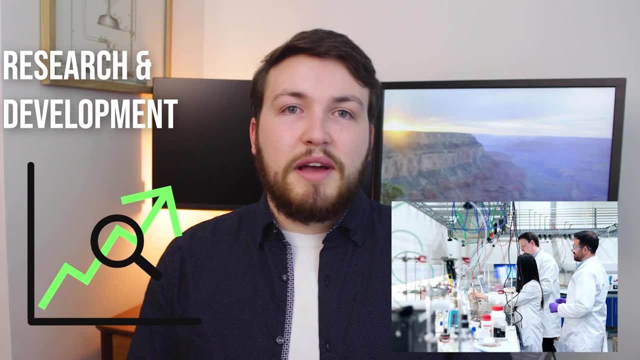 in order to open new windows and new doors for your company. Product engineering can be really volatile as well. You can work on a really big product that's coming out that's supposed to change the game, and then all of a sudden, the company can say: 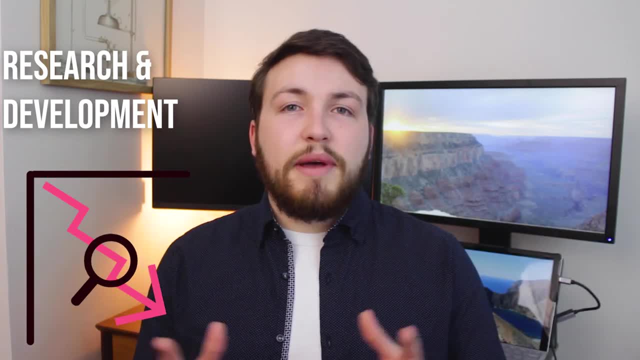 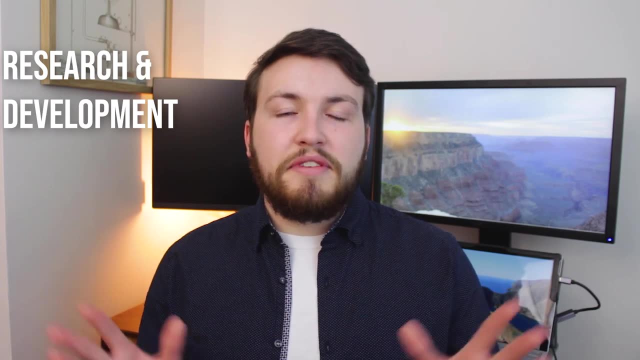 oh well, I don't want to do that anymore because this wind changed direction in the market. In manufacturing, you'll work on a process that's around for 10,, 20,, 30,, 40,, 50 years, And in product engineering, you might work on 50 different projects. 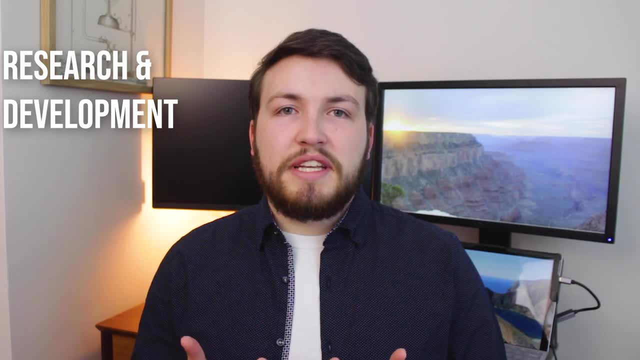 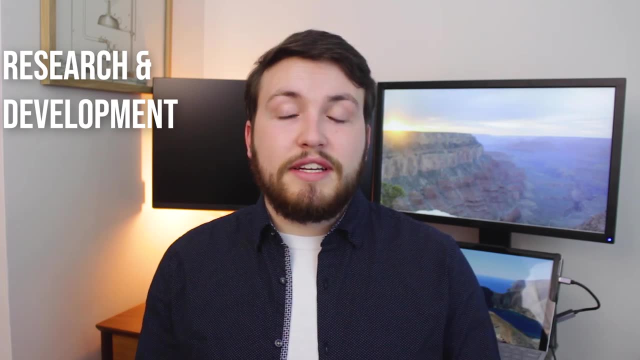 and only five of them will finally be produced. You might spend 10 years working on projects that never come to fruition. Another issue is that most companies are primarily focused on quarterly earnings, and manufacturing processes have a lot of attention because they're directly tied to those quarterly earnings. 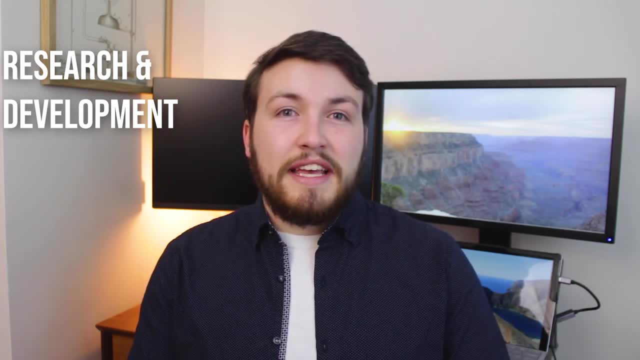 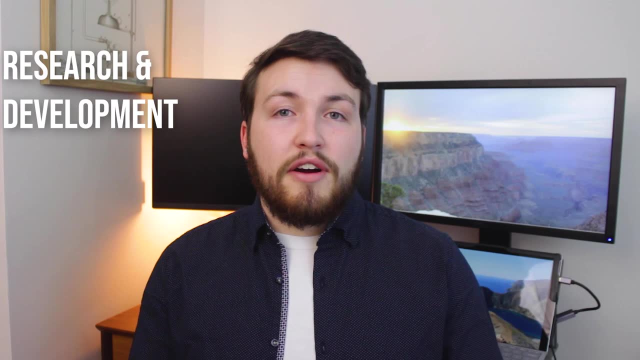 whereas a new product might not touch the quarterly earnings until five years down the line. In the meantime, they're just taking money. So from a high-level perspective, product engineering and R&D usually take a pretty backseat when it comes to chemical companies. 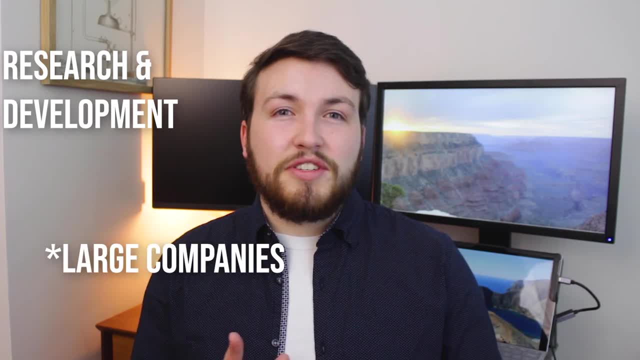 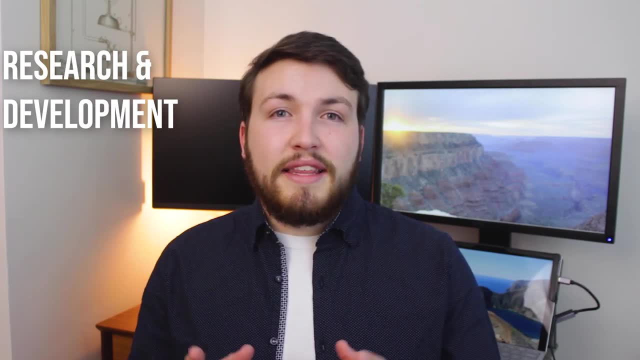 and usually suggest that most companies only put in around one or two percent of their funding into these guys. A lot of these jobs usually are at the startup level because larger companies they don't really want to put in all this money and take on all this risk to build something that might not come into fruition. 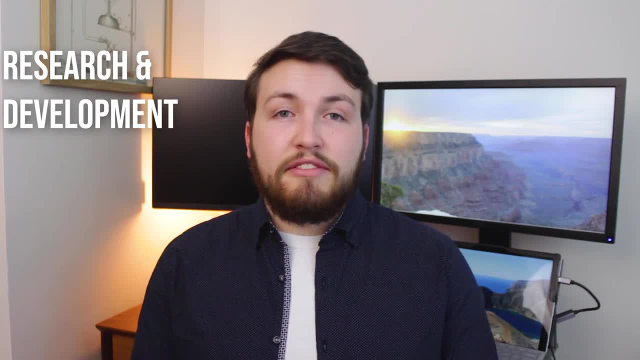 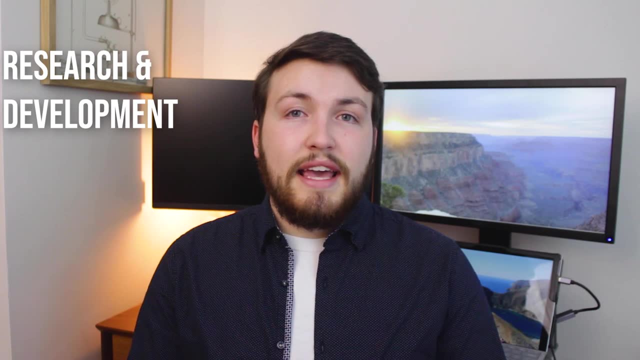 They'd rather have startup companies take on all this risk and then just buy it from them for a really, really high price once they've developed it and proven it in the market. If you want to get into product engineering or R&D, you need to have a lot of experience developing new products. 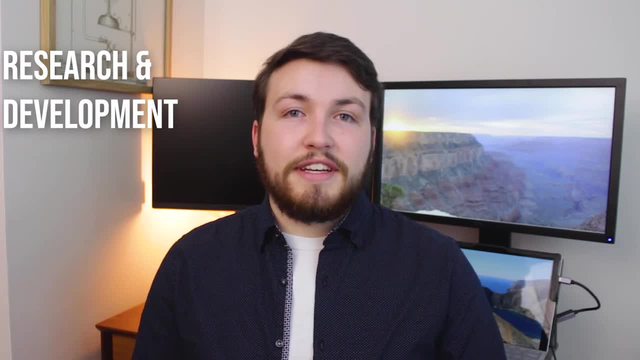 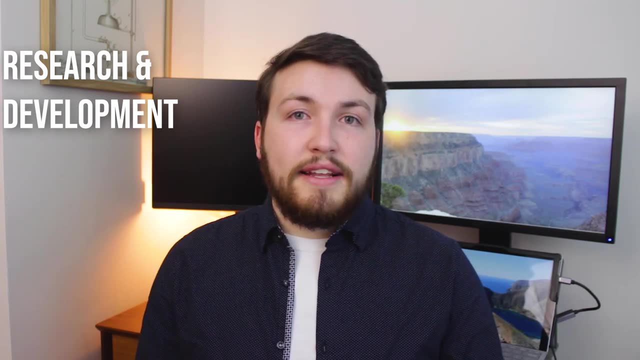 and researching new products in that particular area you're looking at. A lot of times it'll be a process engineer with five or so years of experience, or someone with a PhD, If you really want to manage the most cutting-edge fundamental research in chemical engineering. 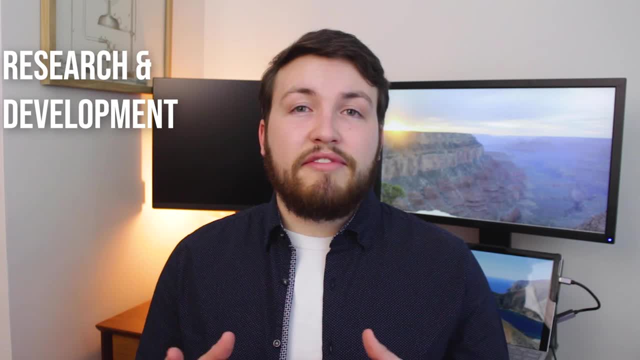 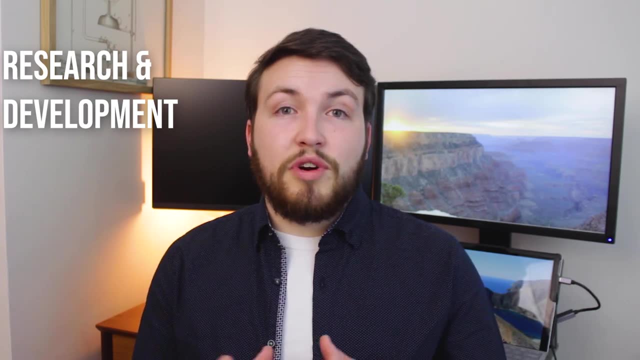 a PhD is pretty much recommended. If you want to work on modifying or improving old products or modifying old manufacturing facilities to make new products, then just a couple years of process engineering working in that environment should do the trick. So I don't want to scare you away from R&D. 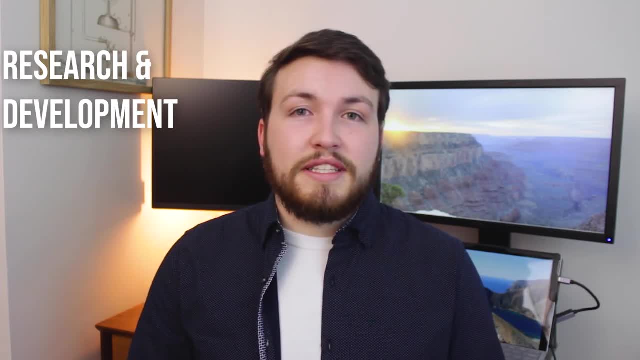 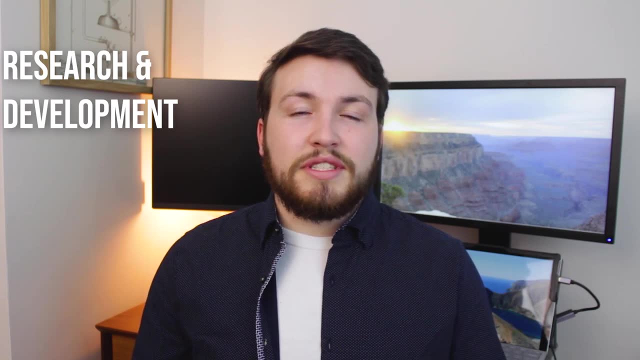 because it's a really fun job and it can be some of the most interesting work that takes place at a chemical facility. But because it takes on such a low priority, they can also lead to lower salaries and a lot more competition. So it's just something to keep in mind if that's something you want to do. 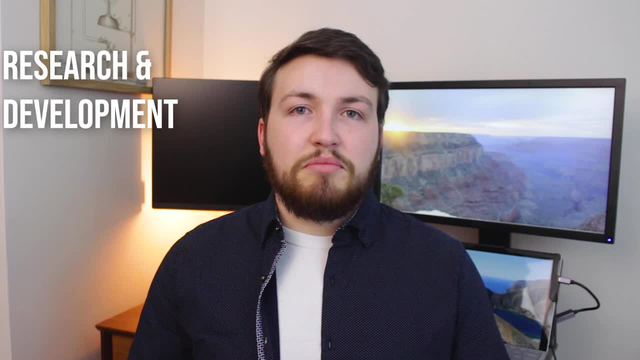 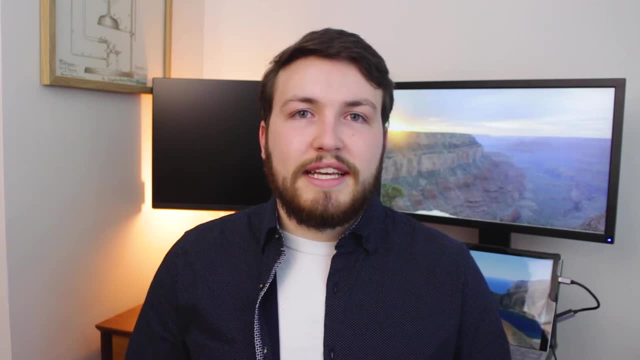 You want to make sure you're well prepared for the role and you have everything in place to make sure that you're successful there. Let's go back to the chemical plant and let's talk about some smaller, support-level roles that chemical engineers can take on. 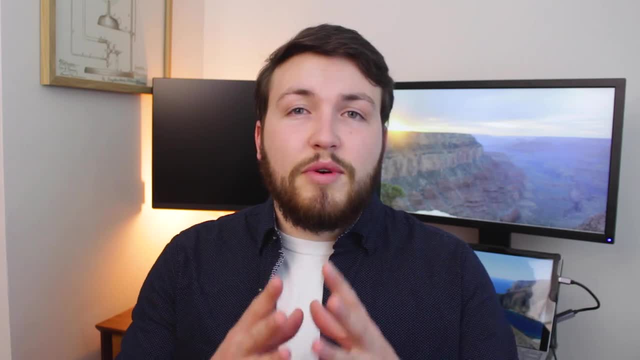 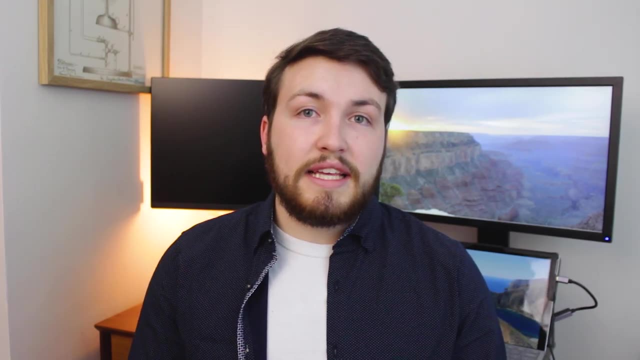 So the proper production and manufacturing of chemicals also requires a lot of different supporting roles that take a lot of technical expertise as well. So process engineers focus a lot on projects and process improvement, implementation of new projects and new technology, but there's also a role called project engineering. 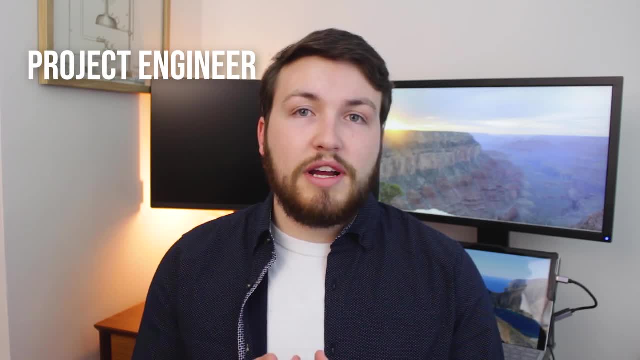 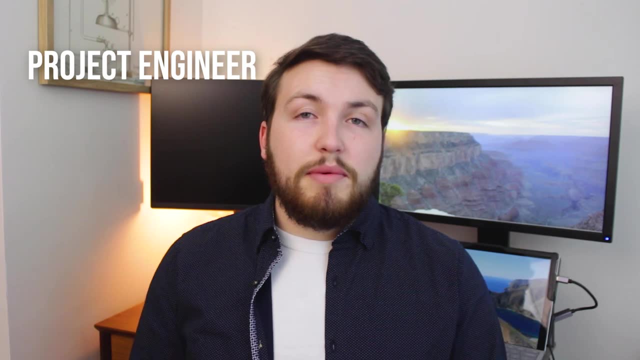 And a project engineer is able to focus just on one project at a time and focus all their efforts on planning and organizing one particular big-scale project. If you want to become a project engineer or project manager at a chemical company, there's a lot of different ways you can get into it. There's a lot of different certifications you can get like Scrum and the PMP or whatever it's called, But the best way to do it is to start off as a chemical engineer in a different role and then move into it. It's usually a second job or a third job. 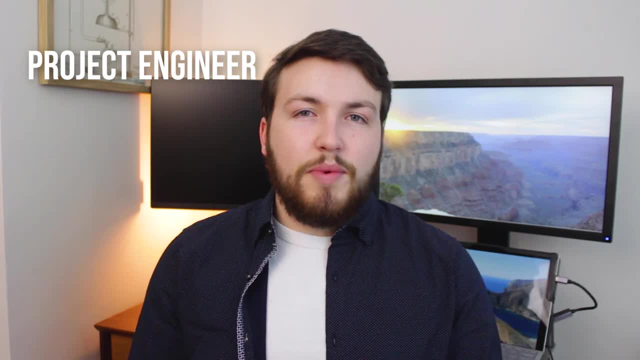 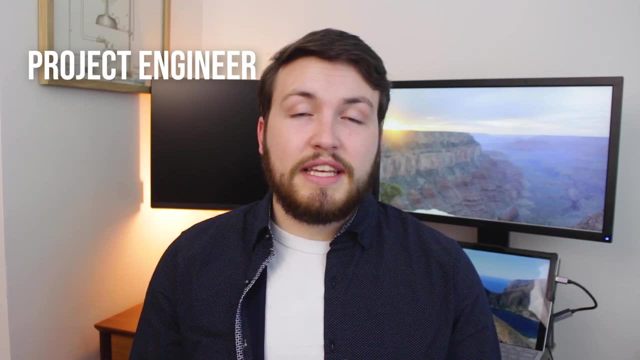 after you've gotten a little bit of exposure to a chemical engineering environment. So why do we need project engineers when we have process engineers who can do that Well, project engineers have more time to focus on bidding out projects, comparing who's the cheapest producer. 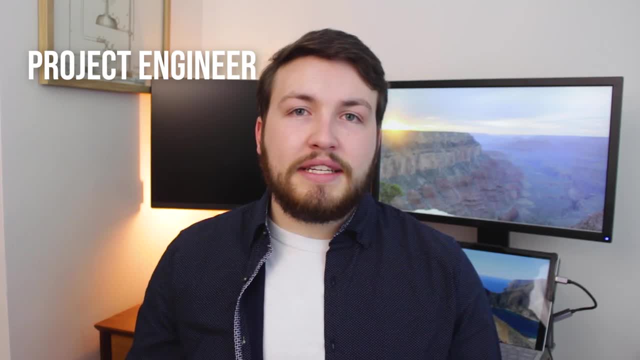 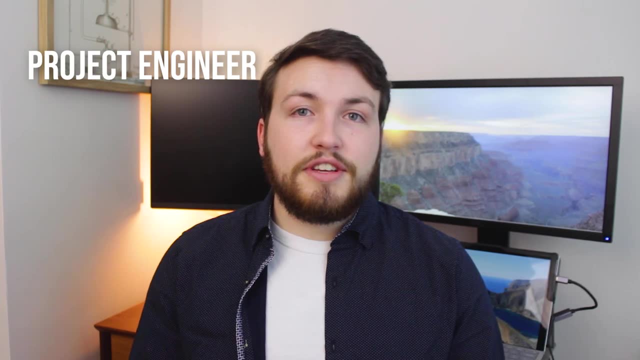 of that particular product you're trying to purchase. they'll spend more time organizing all the different moving parts that come together to make sure a project is within budget and on time as well. Project engineers can focus on anything from a new pump or a new mixer. 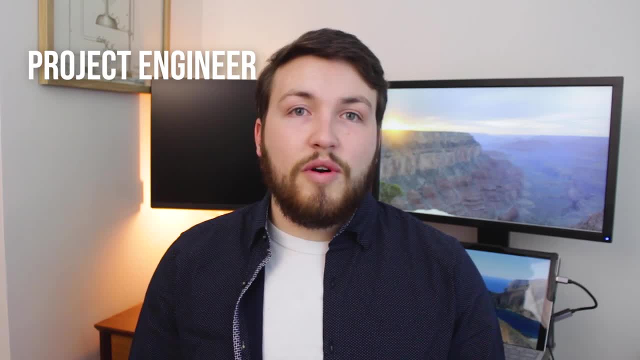 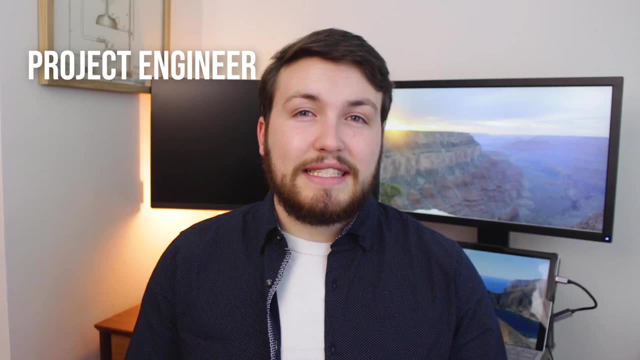 all the way up to a full-on production line or a brand new chemical process. As you can imagine, with a big project on a tight budget and a limited time frame, things can get pretty intense. But this is a pretty cool job and it's a really great way to get into management. Now, management as a chemical engineer can look very different depending on what you're managing, And, as we all know, management, and upper managers especially, get paid really, really well, And it's definitely going to be the highest paying salary as a chemical engineer. 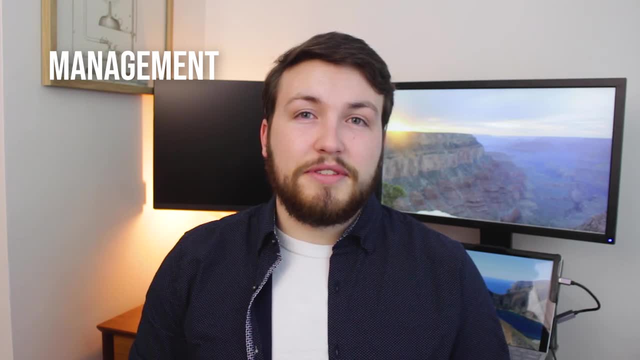 But it's often really hard work and can be a lot of hours. You also have to really really appreciate being a leader and a mentor, because if you don't really enjoy those things, the money's just not going to cut it for you. 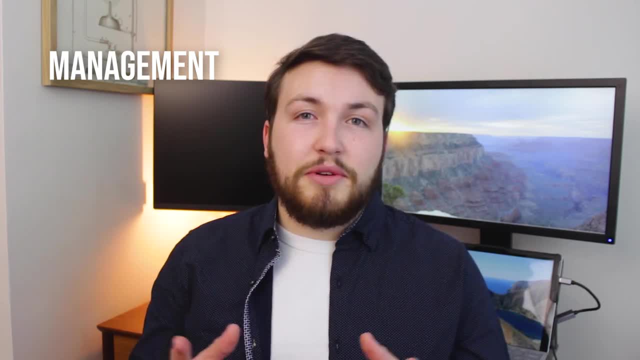 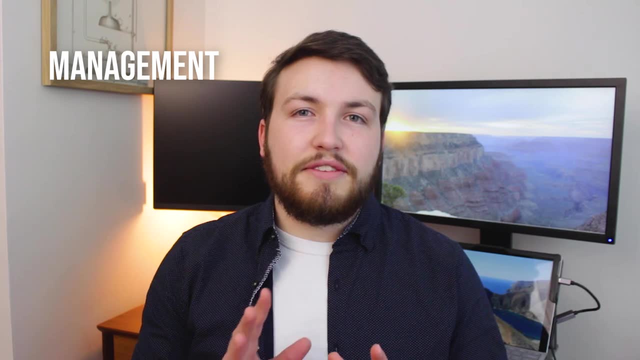 The larger amount of people and the larger amount of money that you manage, the more experience you're going to have to have and the more you're going to get paid. But the role of manager as a chemical engineer can look really different depending on who you're managing. 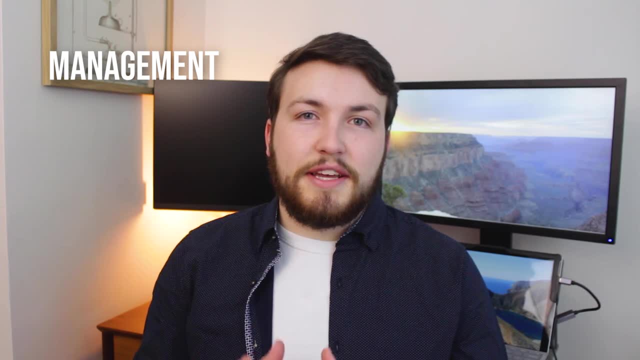 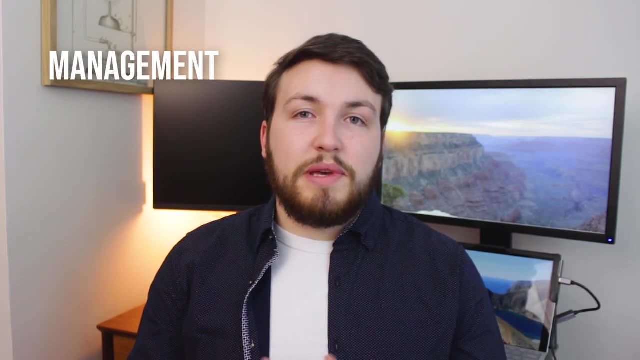 All chemical engineers on a chemical plant are usually managing something. In any chemical engineering role, a chemical engineer is thought of as a manager And they're going to have to manage maybe a process, a few people in a project, maybe a budget. 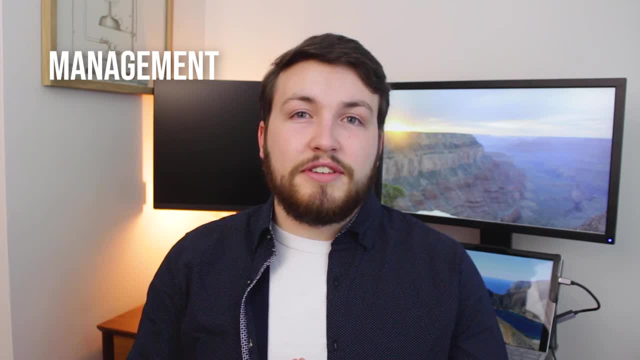 They're going to have to manage something. So it makes sense that most chemical engineers have a clear shot to management if that's what they want to do. Of course, there's a lot of managers that rise the ranks in a particular focused area, like process engineering. 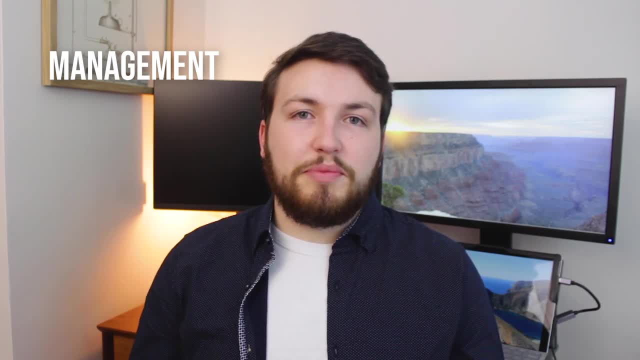 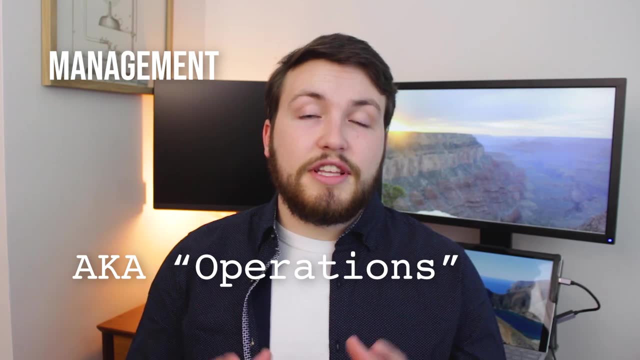 And they'll be a process engineering manager, Or maybe they'll be in maintenance and be a maintenance manager, But the largest group of managers at any chemical plant are going to be on the production side. Managers on the production side are really focused on managing operators and a chemical process. 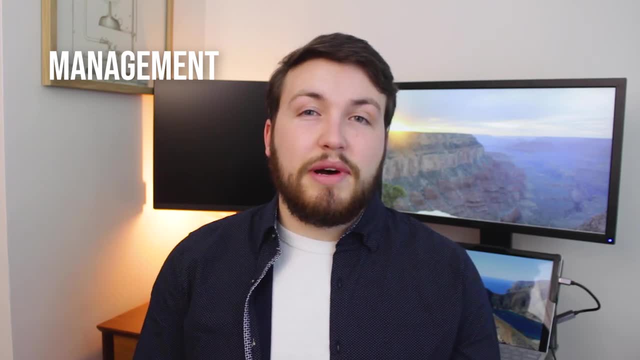 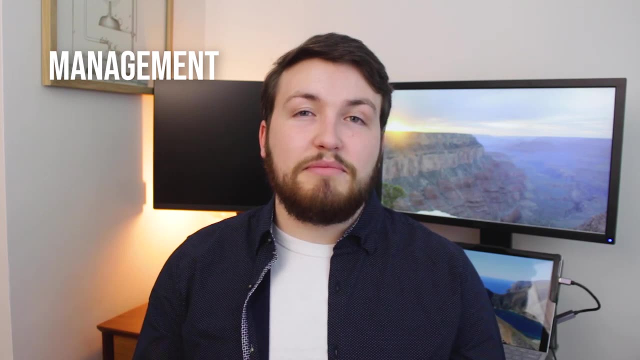 mostly focusing on the money coming out of that process and the budget that's used to operate it. Most chemical engineers who want to get into management usually start off managing a shift of operators- maybe six to ten people- and following them along, keeping up with them. 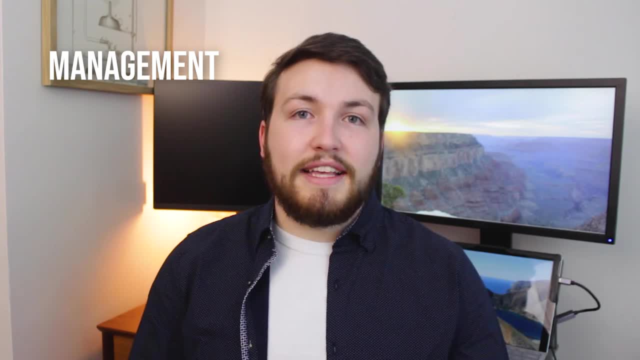 and trying to make sure that they produce the product as intended. Then eventually you might get promoted to managing a whole production line with maybe thirty operators under you and a couple managers, And, as you can imagine, you keep adding on. after that, maybe two production lines. maybe a whole product portfolio. Then you can move all the way up to a plant size management which is anywhere between a couple hundred to a couple thousand people. Just remember that even though this job pays the best, it's also really competitive. It's sort of like a pyramid. 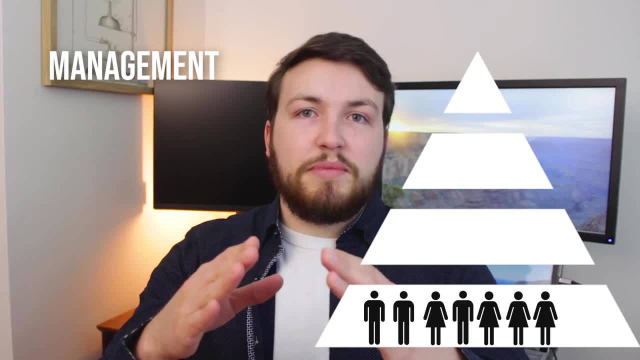 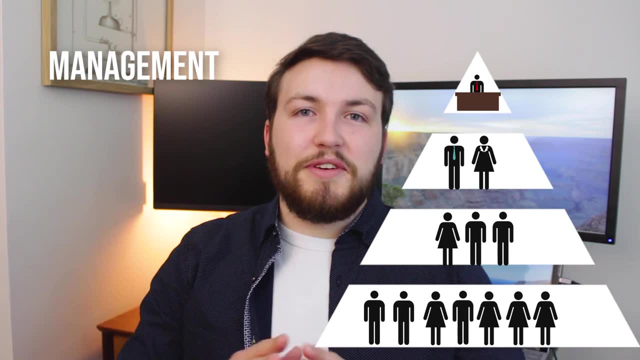 where most of the people are, on the bottom, and as you taper your way up the pyramid, you have fewer and fewer people Until finally, you reach the CEO, who is the ultimate manager, who gets paid the most If you want to be a manager- a good manager- 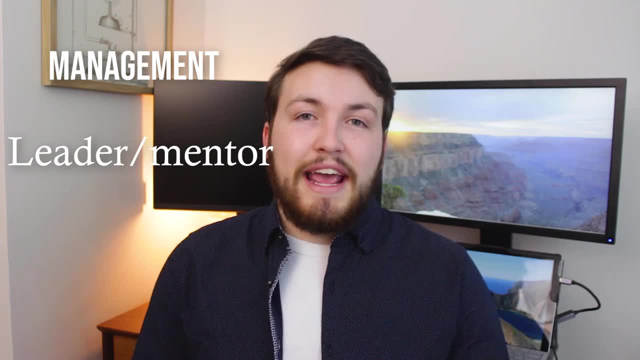 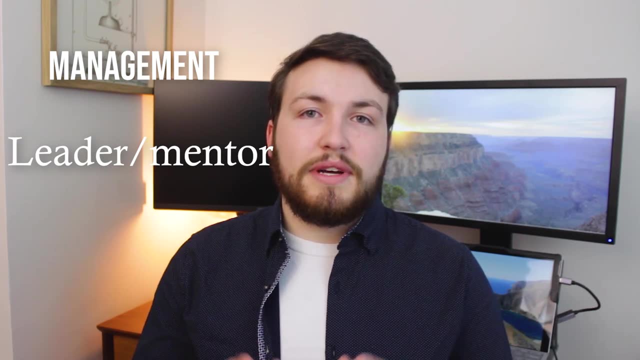 is a leader and a mentor And they're passionate about that. They're a teacher And they're very patient with the people that they're managing. A team and a chemical process are only as strong as their weakest link. So you have to be able to identify. 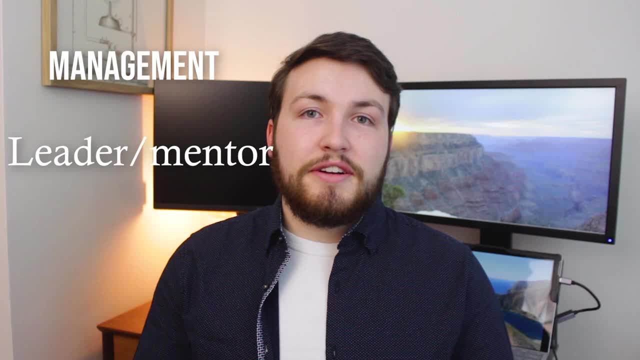 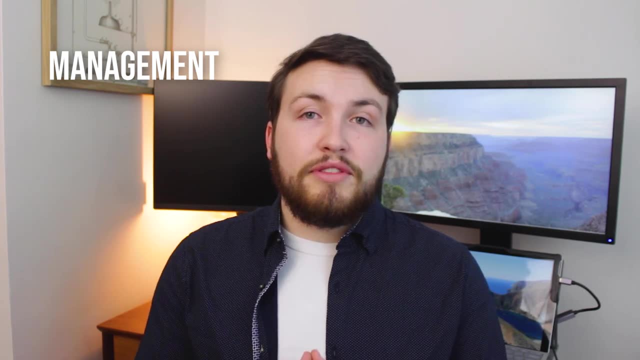 the weakest link, or two or three, and be able to mentor them, monitor them and then finally propel them and coach them to a point where they're as productive as the rest of the chain, if not even stronger, In order to have the right perspective. 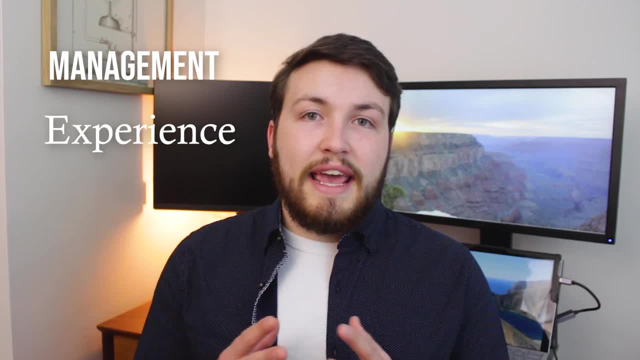 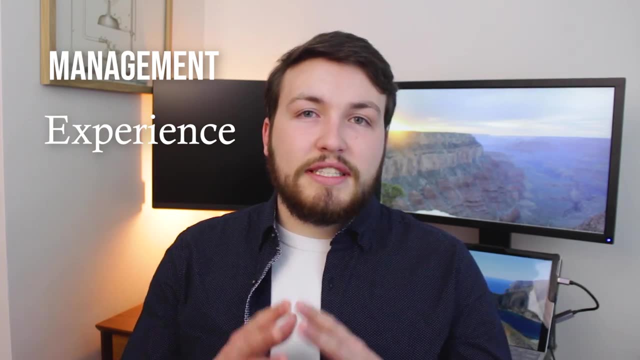 managers have to have also a lot of experience in a lot of different areas, And ideally, a manager should be able to understand how to do each job that they're managing. If you want to work your way into management, I suggest not necessarily focusing on one particular area. 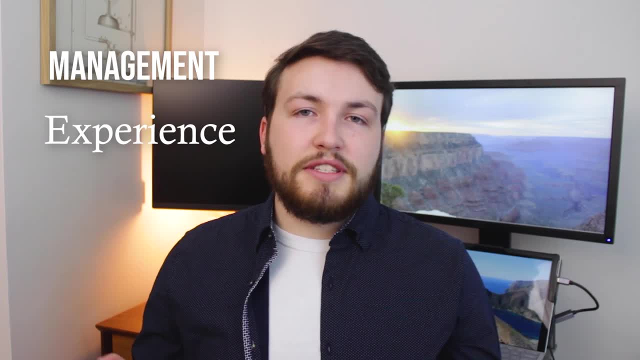 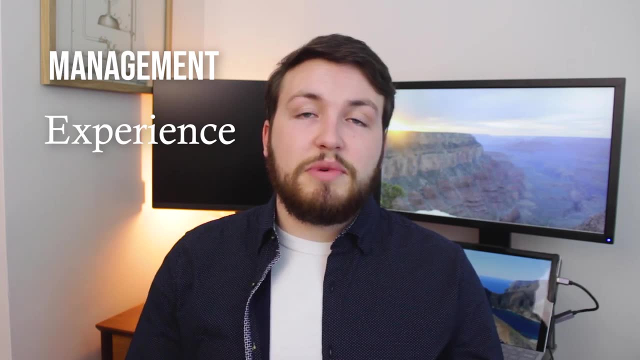 just like managing people, but also collecting a lot of different roles and a lot of different experiences on your resume that can all come together and inform that final manager role. It's not uncommon for upper level managers to have a lot of experience in process engineering. 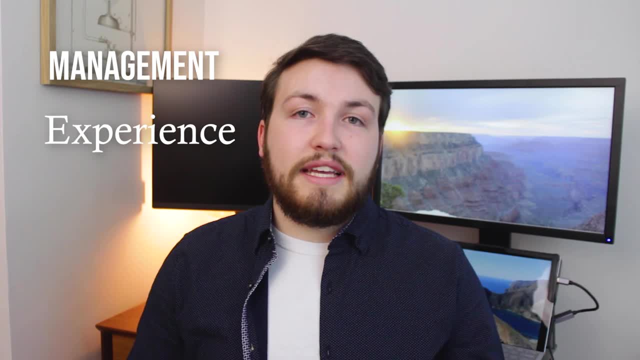 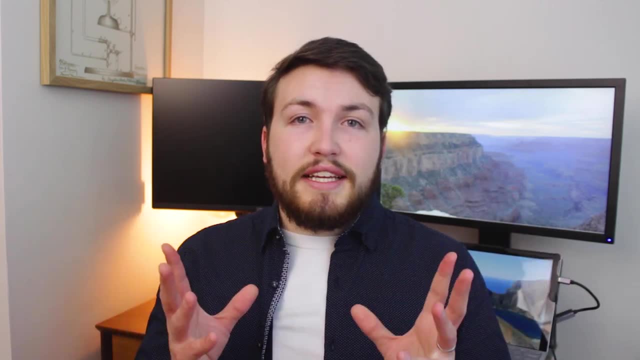 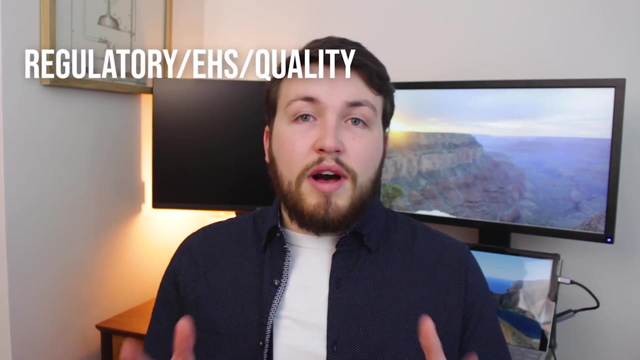 management, environmental, health and safety. quality- A diverse perspective makes a strong manager. There's a lot of roles that mostly just focus on making sure the chemical process is adhering and complying to either external or internal standards and regulatory guidelines, For example, a quality engineer. 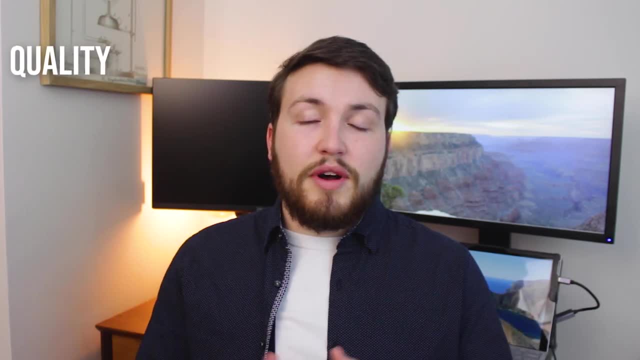 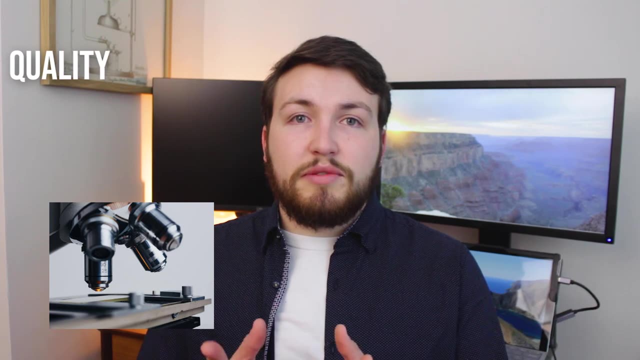 is going to make sure that the process is adhering to their quality guidelines and their quality control parameters. making sure that there's no big issues with the chemical process and the quality of the product it produces. making sure that improvements and changes to the process don't cause any quality issues. 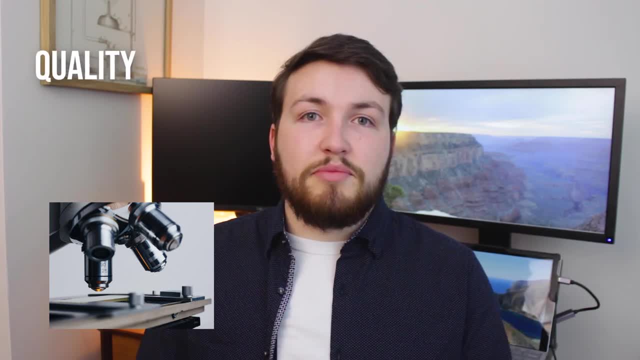 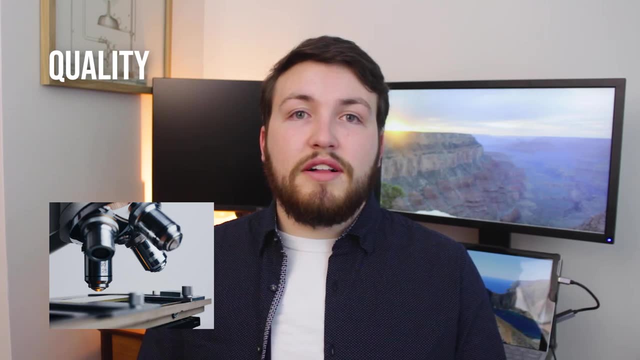 They'll maybe investigate quality issues that have come up in a customer's brought to the company, for example. A lot of new engineers can either start off in these roles or they can get into them later, after being a process engineer for a little while. 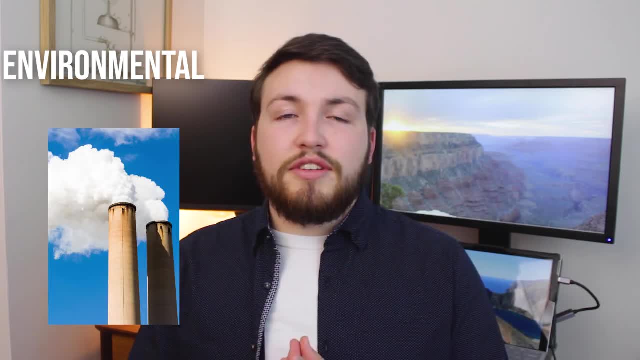 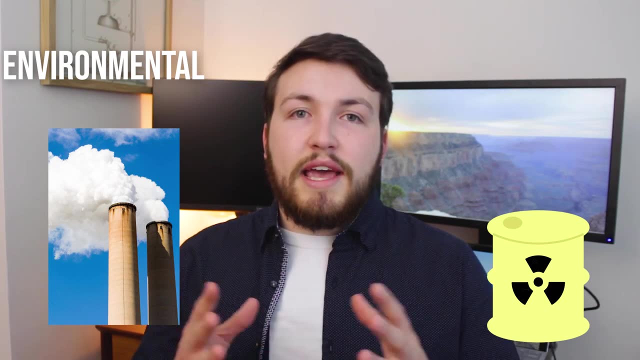 An environmental engineer is going to want to make sure that the chemical company is limiting their emissions, making sure they're not storing more hazardous chemicals than they need to. They're going to want to make sure that the company is complying with all the regulations that are required from the state. 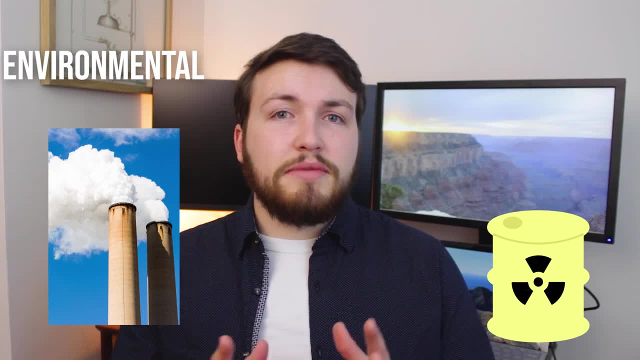 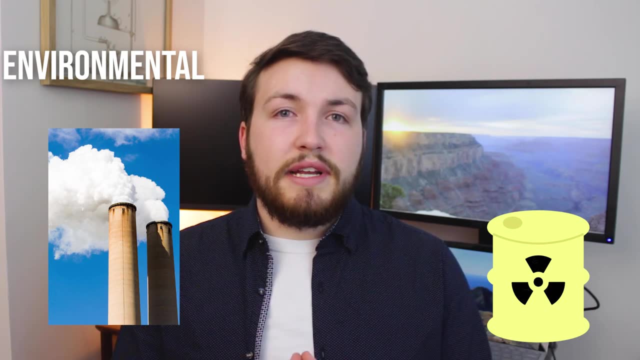 and the country that you're in. It's another one of those roles that's a little more slow going, requires sometimes a little bit more experience, but can also be entered in at the entry level. This support role is all about minimizing the risk that your company has on the environment. 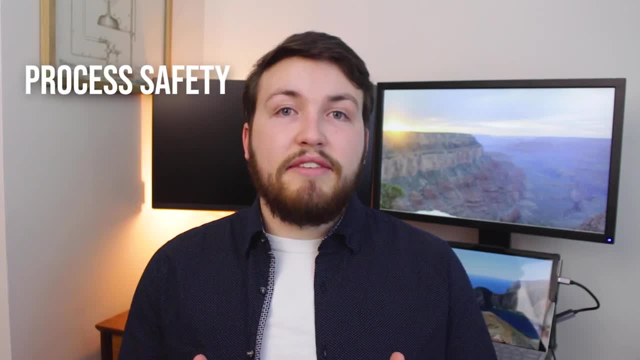 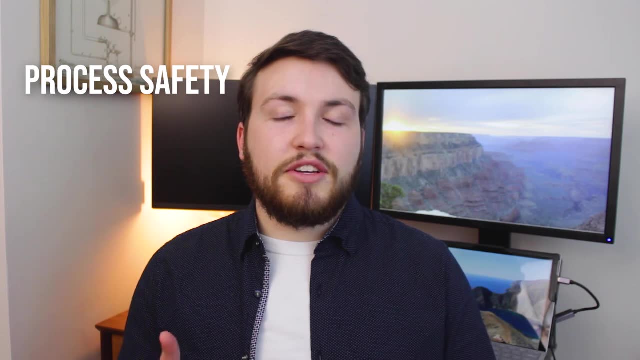 and making sure that they're as sustainable as possible. Next you have your process safety engineer, which is really big for chemical engineers. Pretty much all these guys are chemical engineers and they have to figure out all the different things that could go wrong with the chemical process. 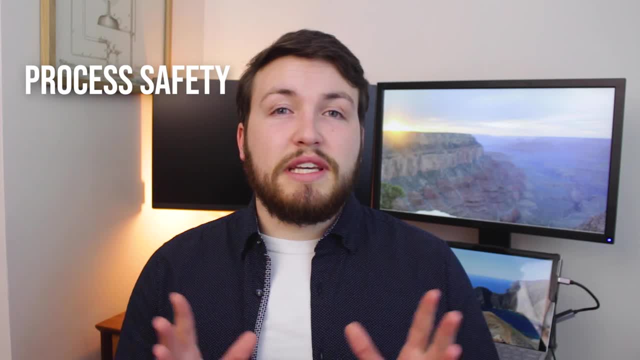 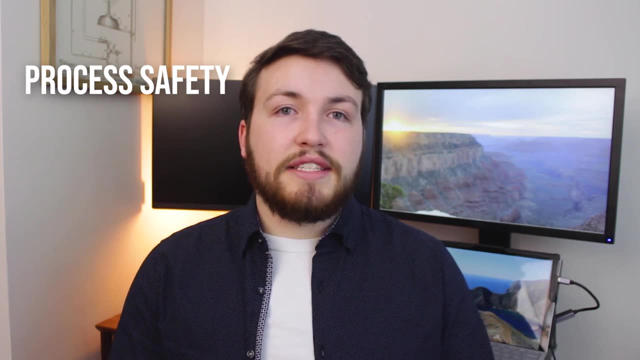 that could lead to safety problems And it's not uncommon for this role to be combined with, or to have a lot of overlap with, environmental engineering. A process safety engineer might specialize in doing what-if or HAZOP analysis on a particular process. They might be a technical expert. 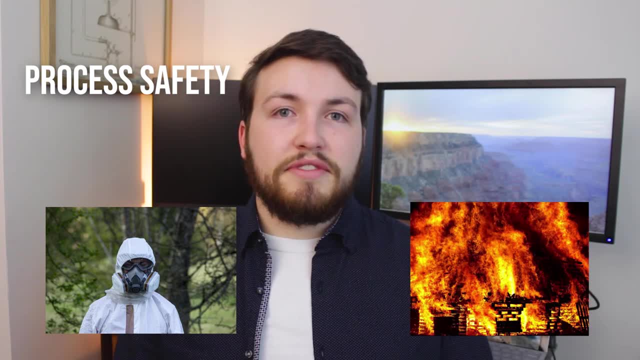 on fire, explosion hazards at an oil and gas facility, for example- And they're mostly focused on minimizing the risk to employees and surrounding communities for every chemical plant that they come across. You're going to deal a lot with OSHA regulations and state regulations, as well as a whole ton of 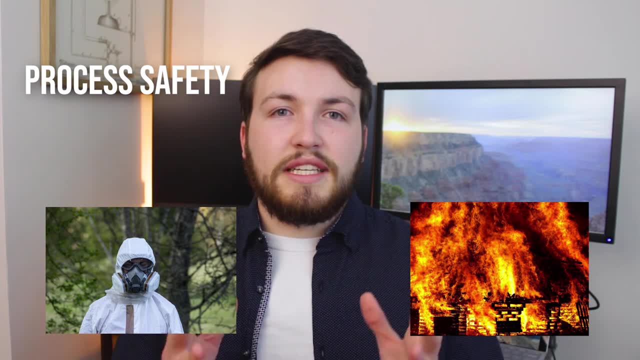 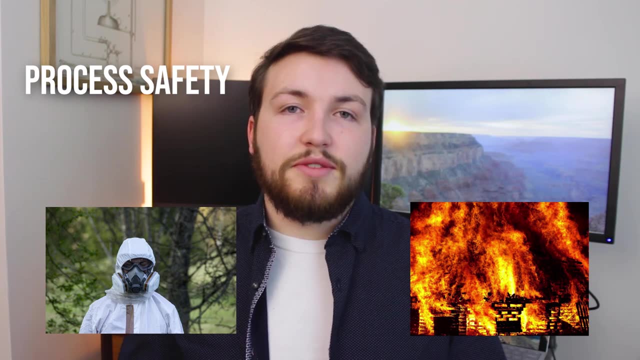 internal codes and standards that your company has put in place in their process safety management system. You can get into this role at the entry level, but usually it's process engineers with a few more years of experience that eventually get into this role. Another supporting role is design engineering. 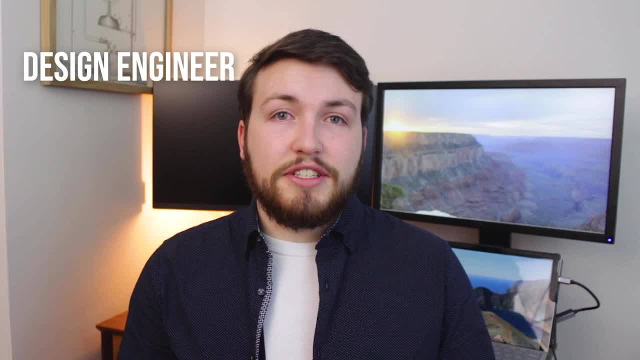 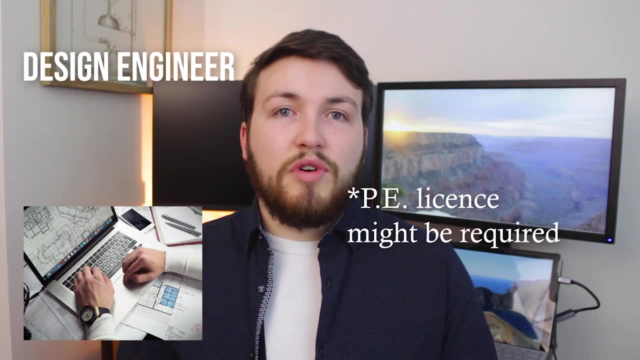 A lot of chemical engineers get into design of new projects and they support project engineers in designing a new tank or a new pump, maybe a new whole entire chemical process. This type of role can be a lot of different things, but usually you're supporting. 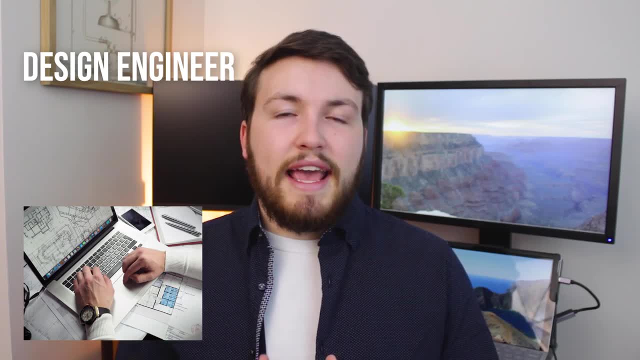 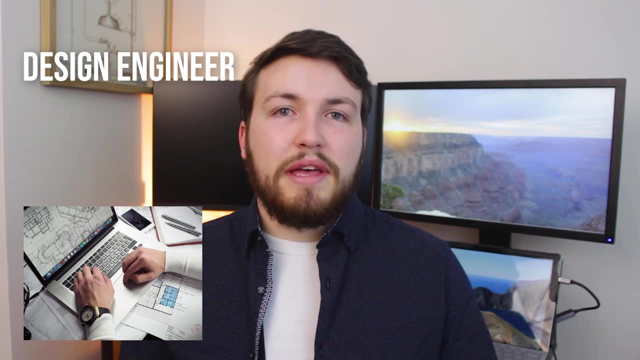 a new project or a new chemical process and making sure that all the math adds up and you're buying the right size tank, you're making sure you have the right flow rates coming out of your pump, you're doing all that design stuff we learned about in school, And that's another great. 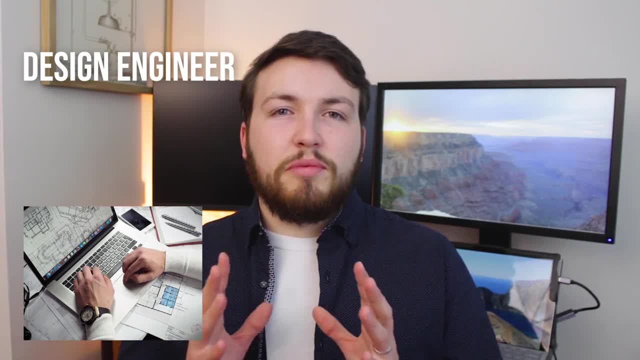 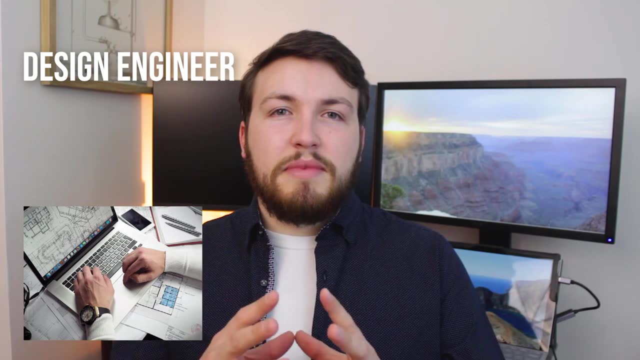 manifestation of the chemical engineering skill set. Every chemical engineer incorporates some amount of design in their work, but a lot of chemical engineers focus on design engineering, which is just focused on designing custom processes for particular chemical plants or particular types of customers, And that can be its. 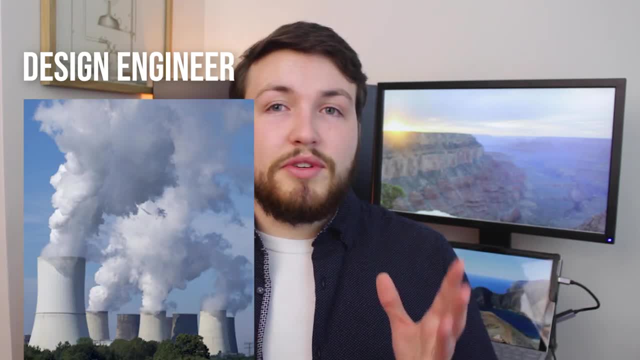 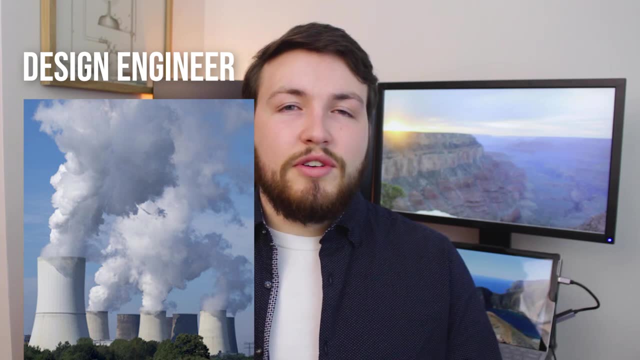 own stand-alone role. Take, for example, a cooling tower company that builds cooling towers for different customers. The customer comes in and they say, hey, I need this sort of flow rate, I need this sort of temperature change. You'll specify a cooling tower. 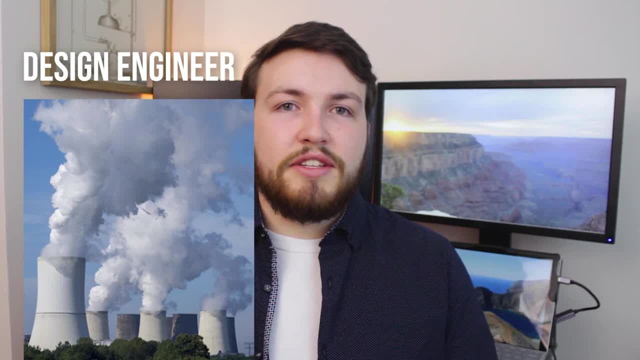 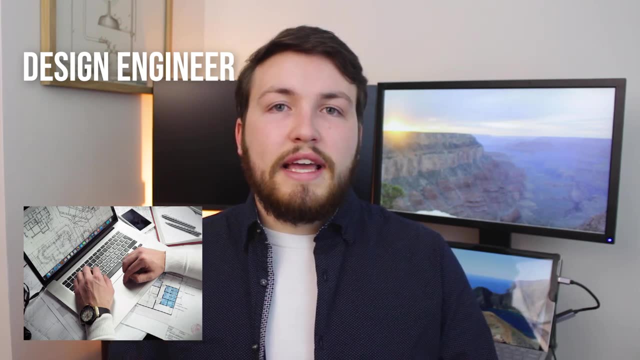 that's best fit for the job, and sometimes you'll even modify your technology a little bit to suit their needs. Design engineering is something that you can get into either at an entry level, starting off as an intern or something, or later on in your career after getting.